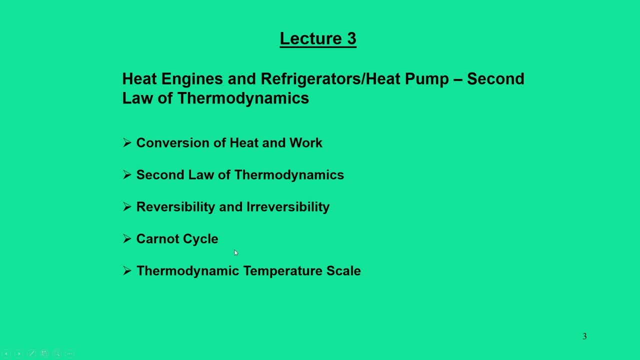 moving further. the ideal cycle for conversion of heat to work is the Carnot cycle. We will try to explain what a Carnot cycle is all about Then, in the last segment, which is the most important inference of Carnot cycle, that is, the interpretation of absolute temperatures. 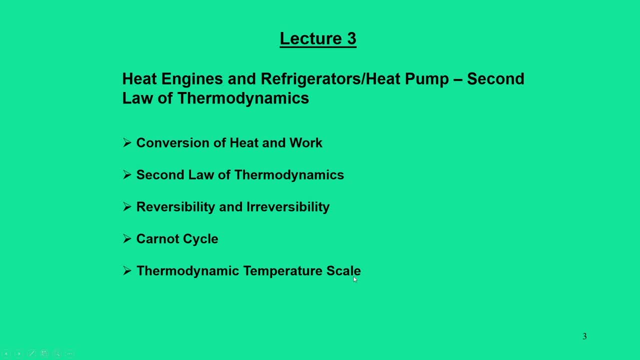 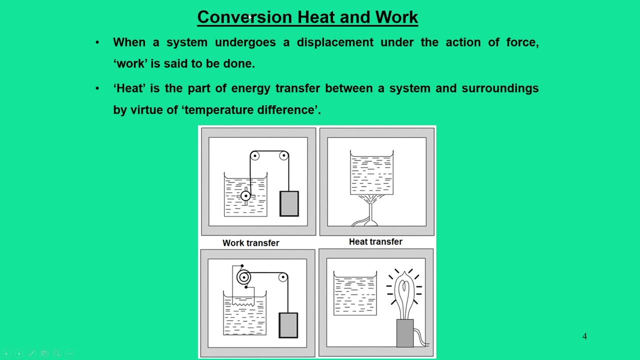 and that we can do it through analysis of thermodynamic temperature scale. So let us start the first segment of this lectures, that is, the conversion of heat and work. So from the first law it says that the work and heat, they can be related together by these. 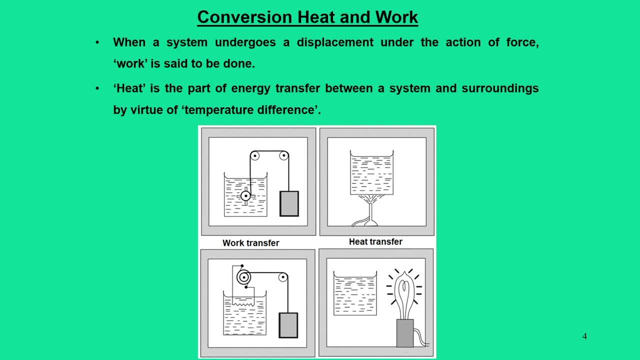 equations, that is dQ is equal to dU plus dW, where work transfer and heat transfer are equal, taken place in a cycles. At that point of time your internal energy is equal to 0. So what we can write for a cycle, We say d? Q is equal to d? u plus d? w, and here d Q is your. 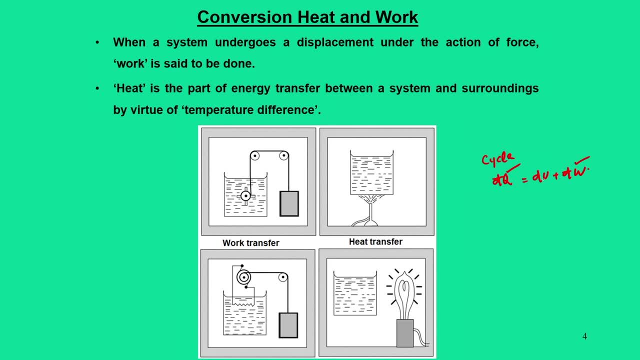 heat interactions d, w is the work interactions d, d, u is the internal property of this system. Now, when in a cyclic process, what happens? The? the starting point and end point remains same. So there is no change in the internal energy. So we can write: Q cycle is equal to w cycle and also we canthis equation also. 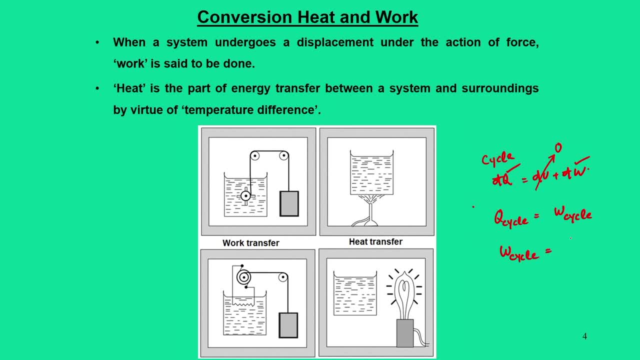 says that w cycle is equal to Q cycle. So these two equations as, although they are meaning wise, they are same, but in terms of interpretation of heat and work they are little bit different. So what it says is that first law does not. 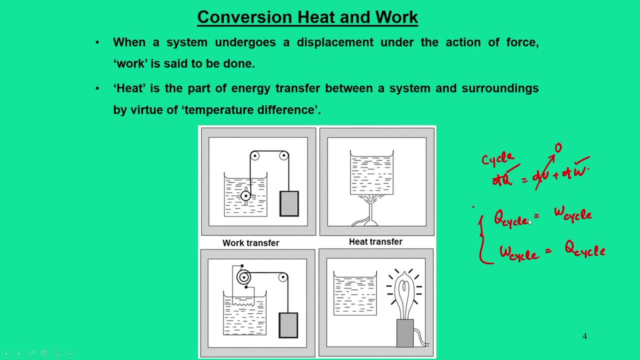 distinguish between the work and heat, but they are interpreted as a energy ah. And when you say w cycle is equal to the Q cycle, it means that complete conversion of work cycle- complete conversion of work is to heat- is equal to w cycle. So it means that complete conversion of work cycle, complete conversion of work, is: 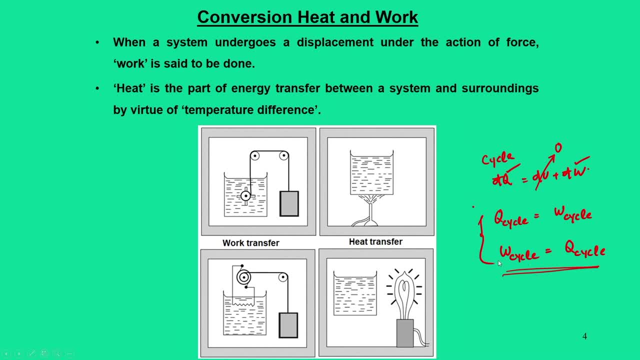 possible. But in other words, ideally speaking, we can as well say that complete conversion of heat to work is possible. but here the first law does not distinguish these equations. Now here we have to make a. f was saying that, why, whether we can write this, both the equations, in a correct way or not? 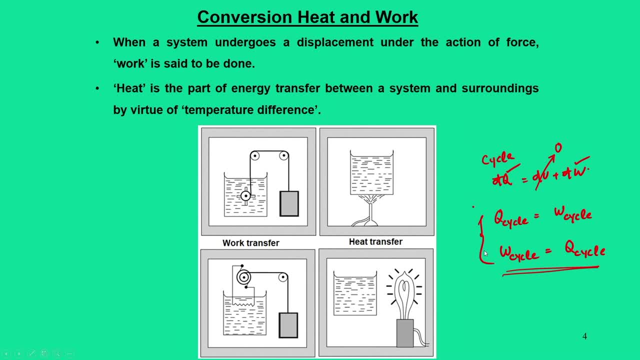 So this turns out to be the interpretation of second law. So in a sense, that when you say heat, so it is by virtue of temperature difference, and when you say work, it is interpreted as the displacement under a action of force. So many a times we view this as a rising 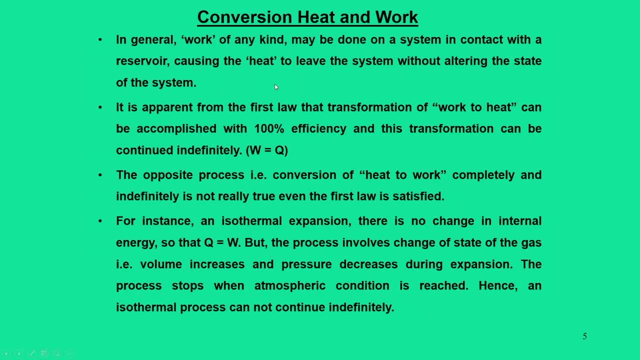 and falling of a weight, Sojust to make some summary of conversion of work to heat. So in general we can say work of any kind may be done on the systems in contact with the reservoirs causing heat to leave the systems without altering the state of the systems. 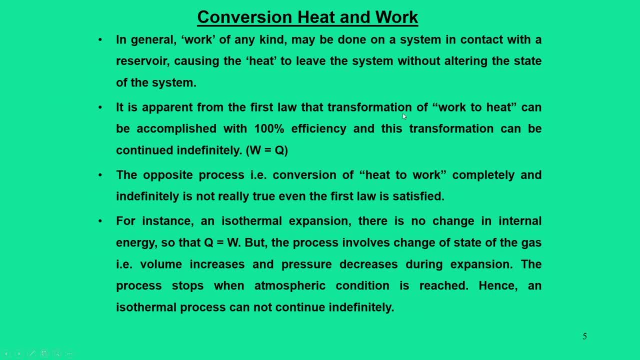 So it is apparent from the first law- transformation- that work to heat can be accomplished with 100 percent efficiency. that is, w is equal to Q And this process can be continue, can be continued indefinitely. That means complete conversion. this process can continue. that means as long as we have. 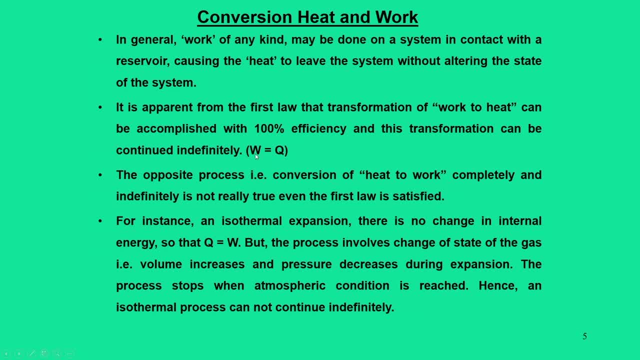 work available to us, we can keep on converting it to heat as as long as this it is available to us. But the opposite process, that is, conversion of heat to work completely and indefinite, indefinitely, is not really true, even if the first law is satisfied. For, for example, we can say in an isothermal expansion process, of course there is no change. 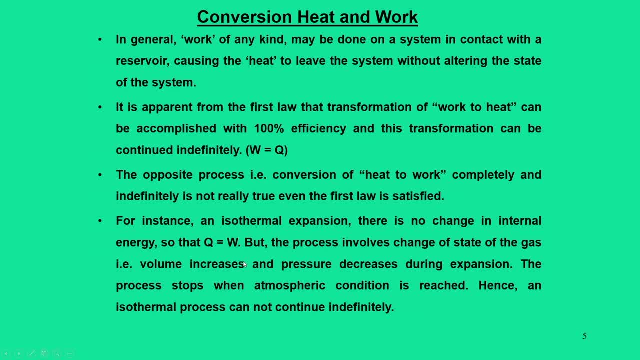 in internal energy because there is no change in the heat transfer. We can say Q is, Q is equal to w And the process involves change of state of the gas, which means that that means an isothermal expansion. temperature remains same, the volume increases pressure. 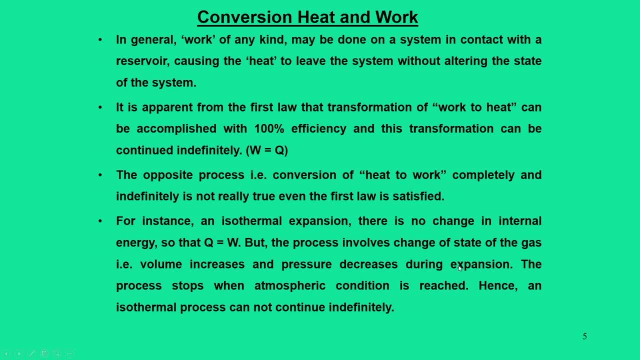 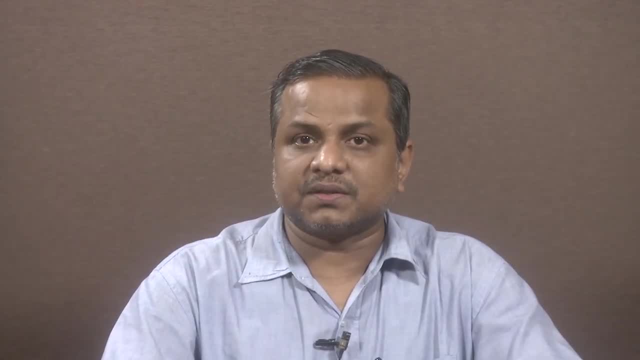 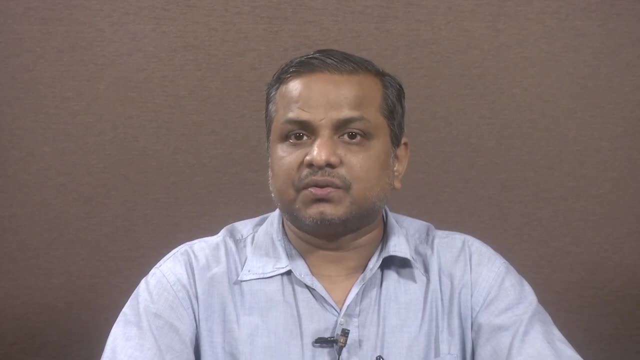 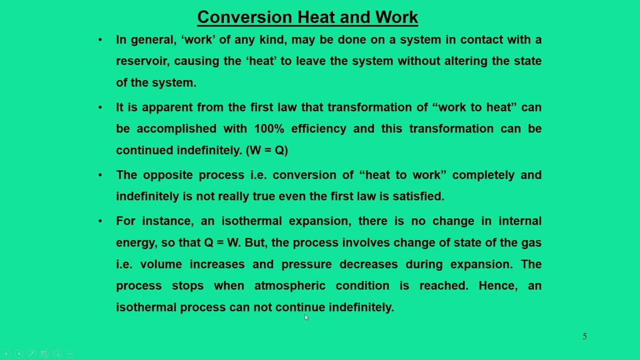 decreases. decrease of pressure is possible till one particular point. For example, in this case the downstream atmospheric conditions restricts this expansion process. That means pressure can be decreased continuously to the dead state atmospheric conditions. So in other words we can say that isothermal process cannot continue indefinitely. it has. 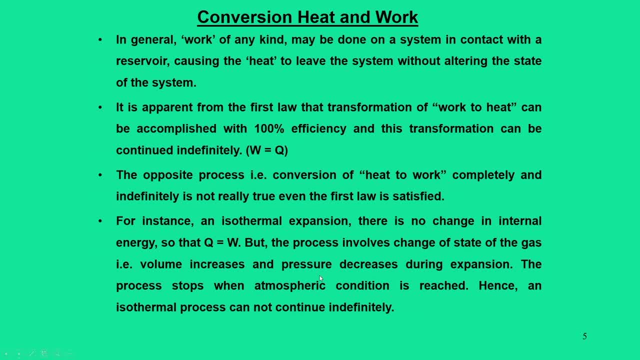 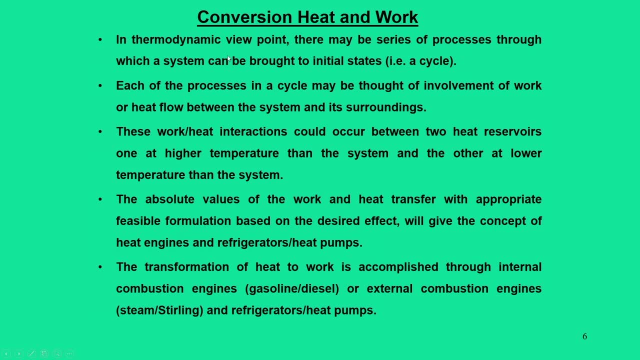 to stop somewhere. ah, So this, this is the conditions thatFast law does not identify this concept. So in a thermodynamic viewpoint, we can say that there may be series of processes through which the system can be brought to its initial state. that is, cycle and each process. 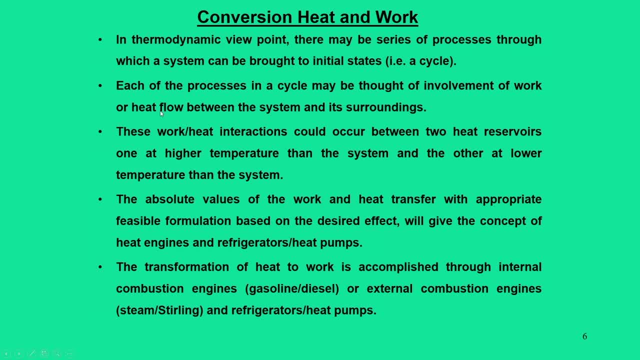 of the cycle involves the involvement of work flow and heat flow from the system and the surroundings. So work interactions or heat interactions can occur between two reservoirs which are maintained at two different temperatures: one at higher temperatures, other at the low temperature of the systems. ah, So this concept was told, that when, if you want to transfer thework, 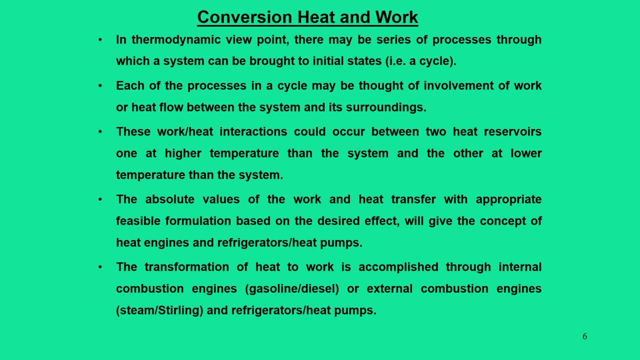 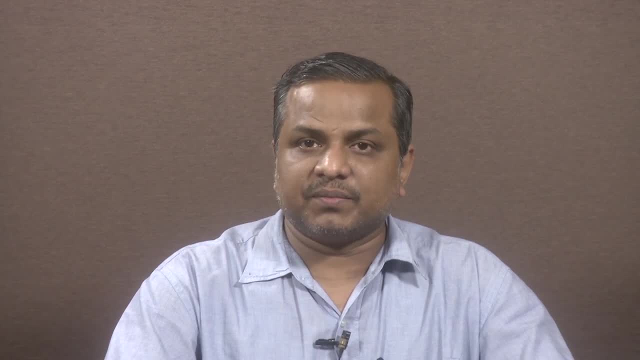 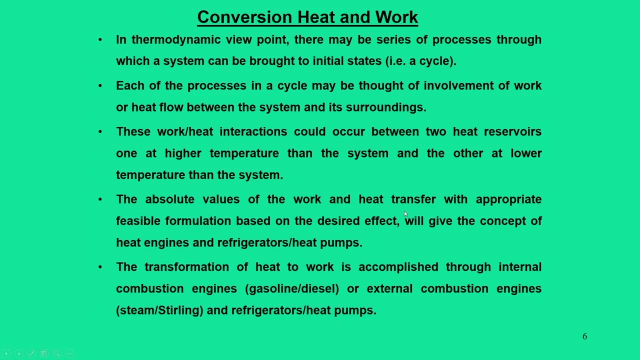 interactions from heat, then you have to view it as a as a cyclic process That should occur between two temperature limits, that is, at high temperature and lower temperatures, And the absolute values of work and heat transfer is based on the type of feasible ah feasibility of the formulation of power requirement. So this gives the either. 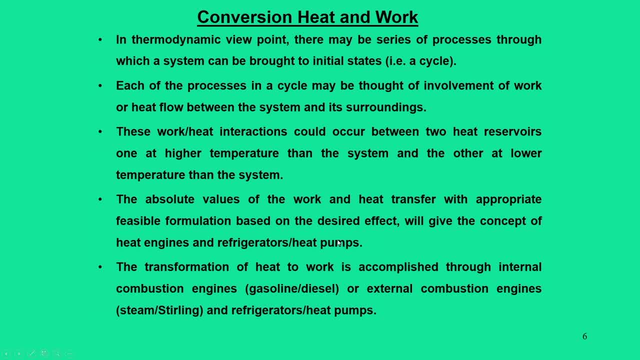 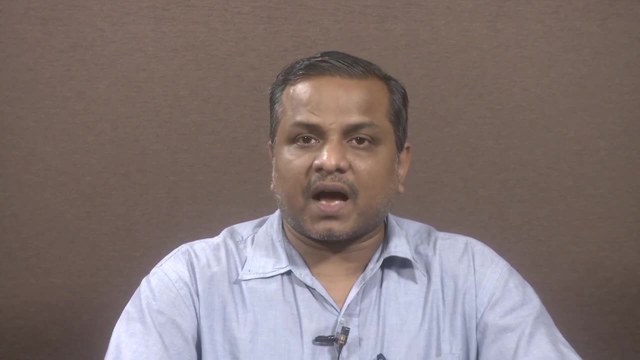 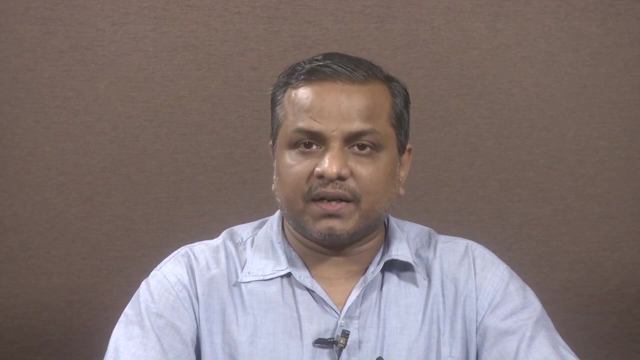 concept of heat engines, refrigerators or heat pumps. Nowfrom the second law, which we will be talking later, That when we, when you talk about conversion of heat to work, it is accomplished through ah, through a device, and or is, or you call it as a cyclic device and in our term we call 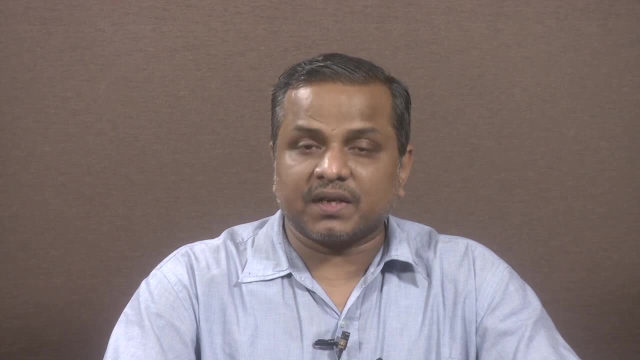 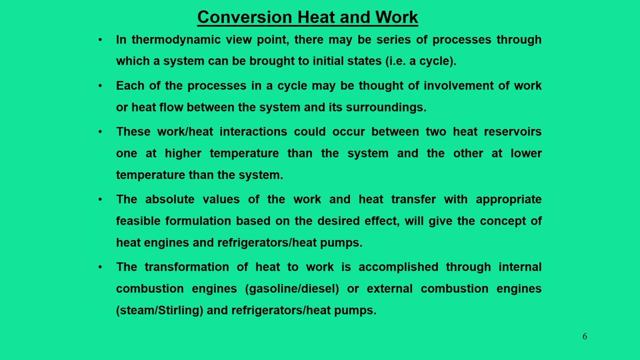 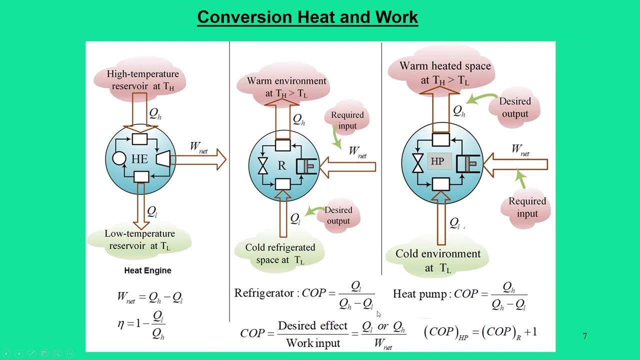 this as a engine. So this engine could be an internal engines, internal combustion engines like petrol engines, diesel engines or any kind of external combustion engines like steam engines. So that is, and we have a heat engines. that means, in order to transfer thein order to 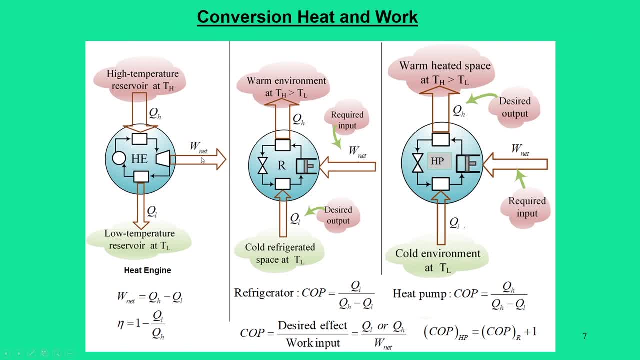 have a net effect of work- transfer from heat to work- then we must haveintroduce an, a cyclic device, And this cyclic device we call this as a heat engine. it must takes Q- H amount of heat and reject Q- L amount of heat heat to the low temperature reservoir. So in 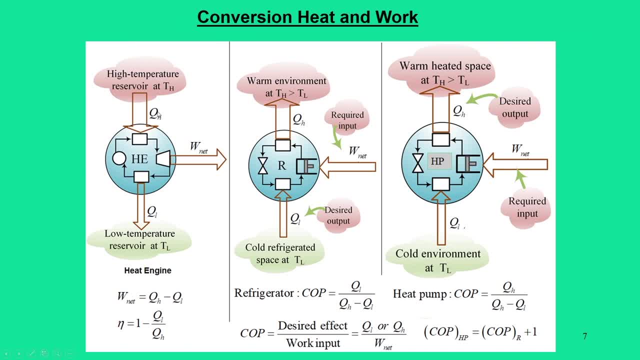 the process. if you can justah transfer The look into itsfirst law analysis, then you can say: net work is nothing but difference in the Q H and Q L, and from this we can also derived the expressions for efficiency of this heat engines. that is nothing buta ratio of Q net by Q H. So this turns out to be: 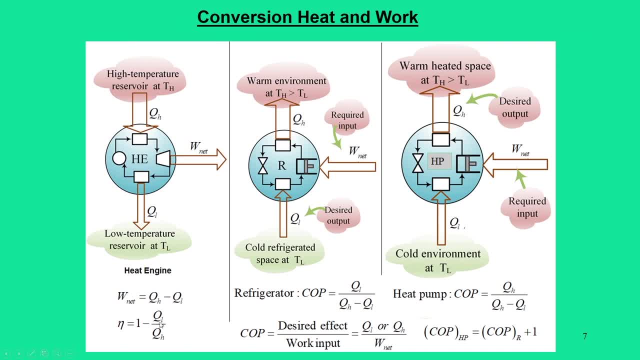 efficiency of this engine, heat engine- is 1 minus Q L by Q H. So this is one concept where we call this as a power producing device, where work is comes out of the systems, that means a work is done by the system. Now, in other situations, what other two situations? what we have is that 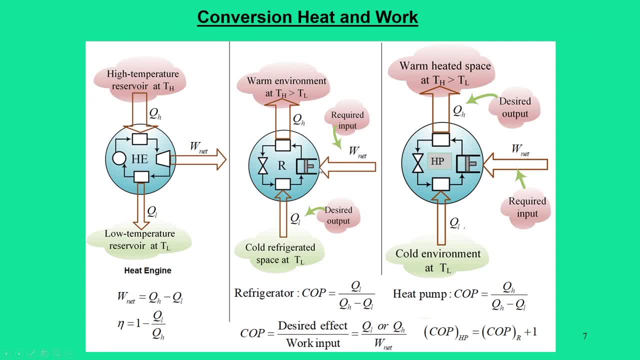 work is being fed into the systems and side by side. if you do this, then this particular cycle- heat is in cycle- can be reversed. one is that means heat can be taken from the cold, refrigerated cold space and we and and it can be rejected to warm environment. 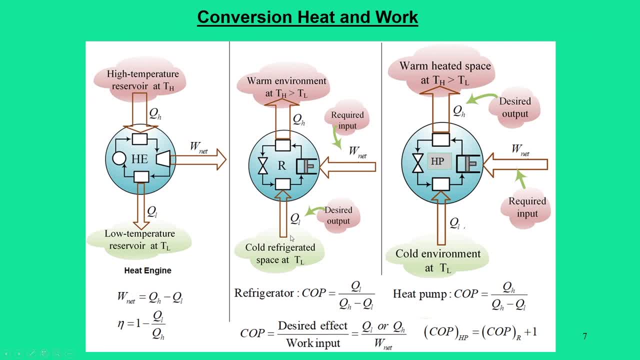 So in this casewhen if you, if, if our- in other situations also similar concept is there, but that depends on the. in both the cases we have the required input is W net, But the desired output is different. if you or if you are concentrating on the, the desired 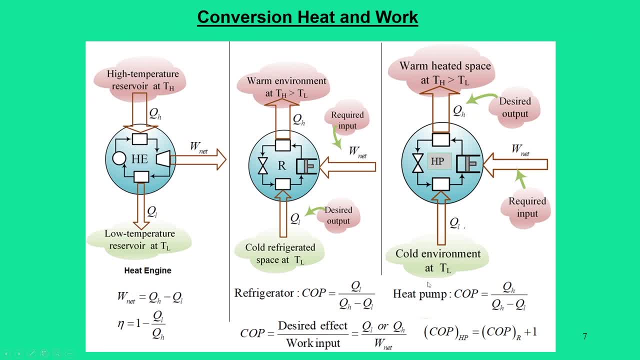 output as Q H, then such a philosophy, we will call this a heat pump. If your desired output is your Q L, that means Q L is the essence of your requirement, and so we is call this as a refrigerators. So based on this, we derive the expressions force, coefficient of 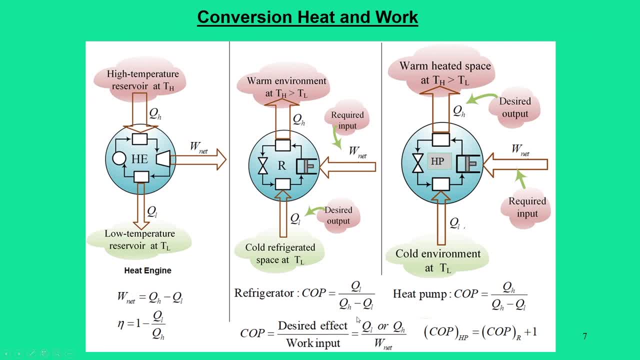 performance. that is Q, L to H, So Xう λandan. Since the heat pump will be used for that cm as a temperature and pressure value, the inner squares will also be commissions, So L by W net. So same same expression we can use in the other in a different form, that. 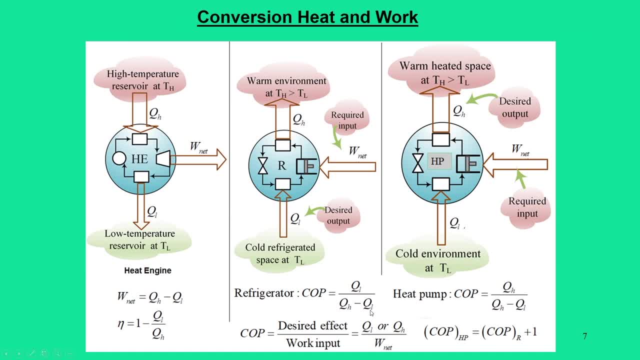 means q, q h minus q L is nothing but your W net net amount of work which is done on to this systems. Other concept: we can use it COP as q h by q h minus q L. So this is the three situations where we have demonstrated that how conversion of heat to work is possible. 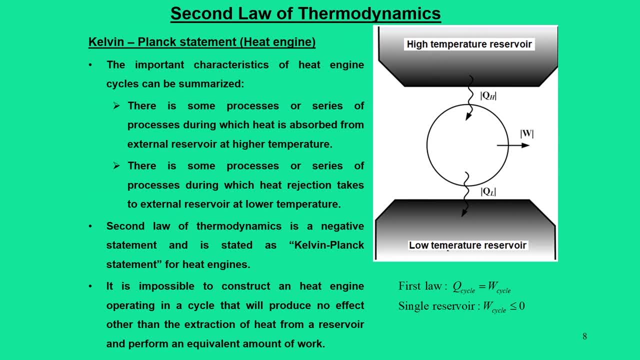 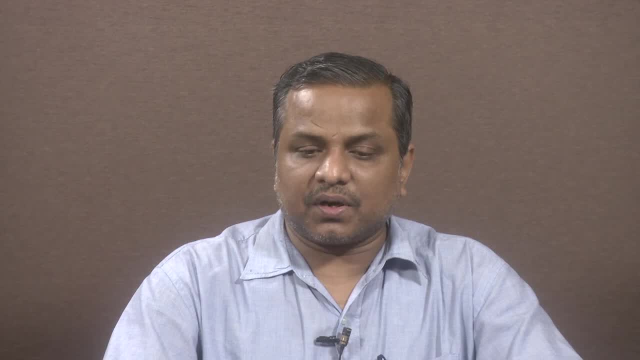 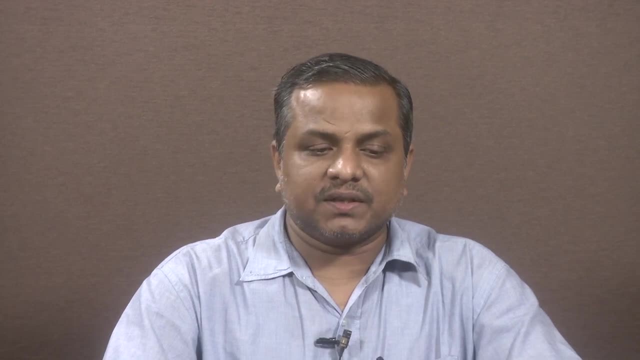 And these concepts leads to the fact that is called as second law of thermodynamics. So this in a, when you talk about the second law of thermodynamics, there are two possibilities or two important statements. One is Kelvin Planck statements, other is Clausius statements. So let us talk about 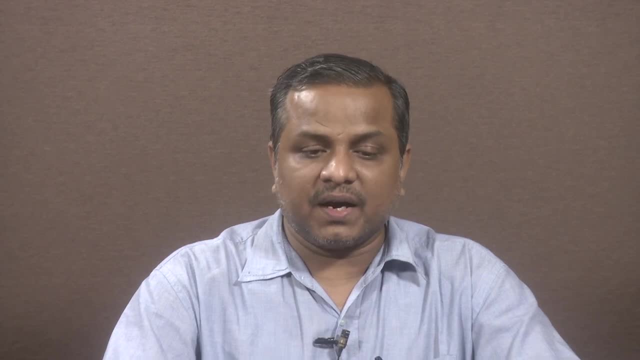 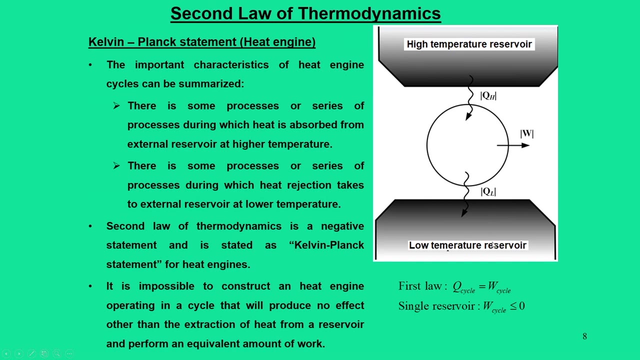 the first statement, which is Kelvin Planck statement, and it is based on the concept of heat engines. So, essentially, we have a high temperature reservoir, we have a low temperature reservoir. So if a heat engine has to operate in a cyclic manner, thenwe can say: the heat. 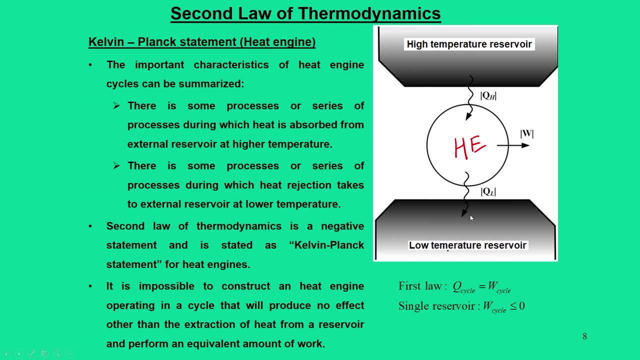 engine takes heat, So Q H amount of heat, and rejects Q L amount of heat to the low temperature reservoir, and side by side we get a W amount of work. Now one interesting one, one. one of the interesting feature is that when you say that the process has to occur in a very, in a slow manner, then 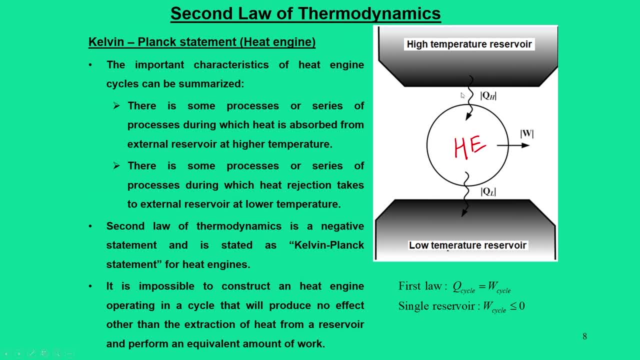 we can view this particular things as a reversible processes. ah, So what we can have is that when you take this amount Q H amount Q H- amount of heat, we assume that temperature of hot reservoir should not drop. That means this particular temperature T H of the hot reservoir remains as it is, and the process 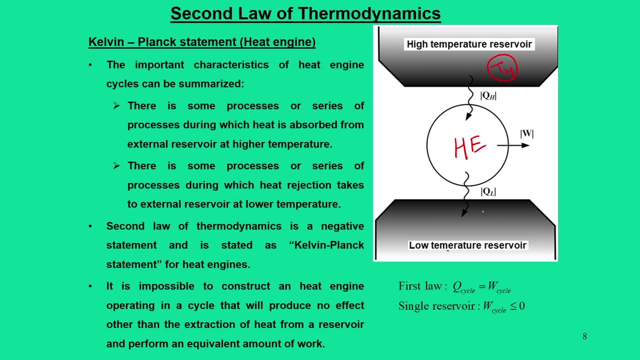 has to take take place in an isothermal manner. Similarly, when we reject the heat to the low temperature reservoir, that is, T? Lthen the, the temperature of this low temperature reservoir should not change. So this, all these processes, has to occur in a isothermal manner. So that is what we 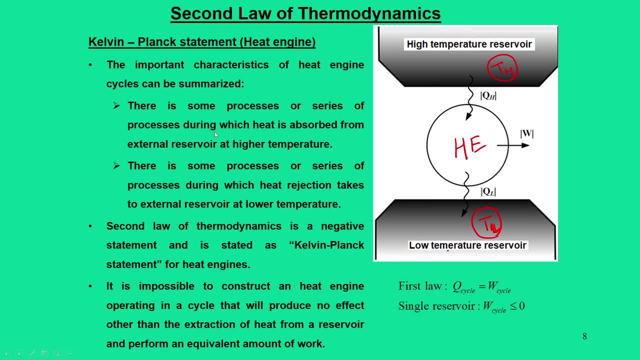 say, there is some processes or series of processes during which heat is absorbed from the external reservoir at higher temperatures. There are some series of processesthat occurs for which the heat rejection takes place external to the external reservoir, at lower temperatures. Now, here and in this process, what we can say based on the first law, we can say cyclic. 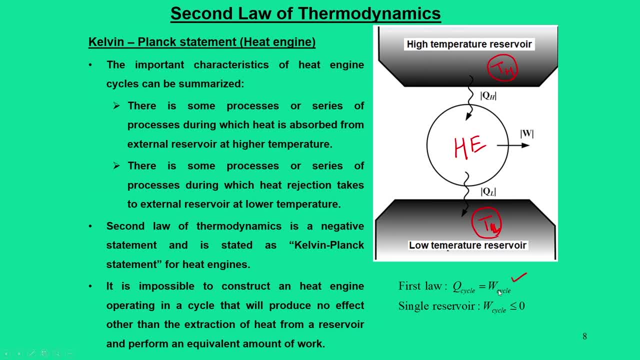 heat transfer. Q cycle is equal to cyclic work transfer, that is, W cycle. And one of the important thing is thatif the here- here I will try to say that- if there is no change in the internal energy, then we can say thatthe first law is satisfied. that means Q cycle. 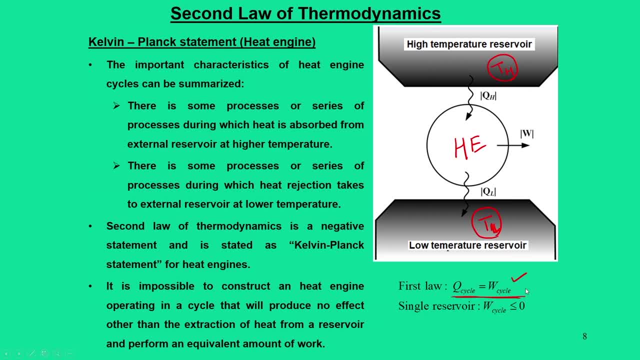 is equal to W cycle. So whatimposes the second law? is it possible that all the Q cycle is equal to W cycle? So here thethe second law imposes the conditions that W cycle should be less than or equal to 0. So in other words, we can say thatthis this W cycle either can be 0 or it can be. 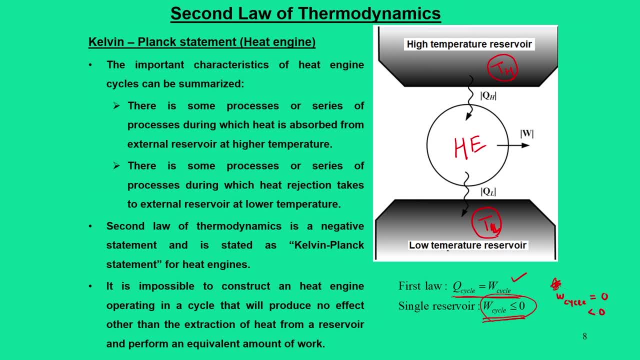 less than 0. So less than 0 means that some part of heat must be rejected to the low temperature reservoir. So with this condition of impositions we can write the second law of statement in a negative form, that is, it is impossible to. 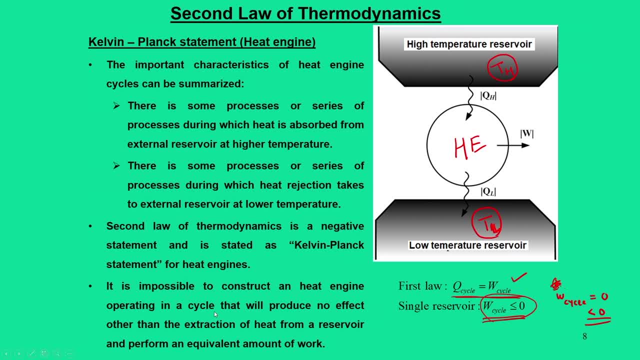 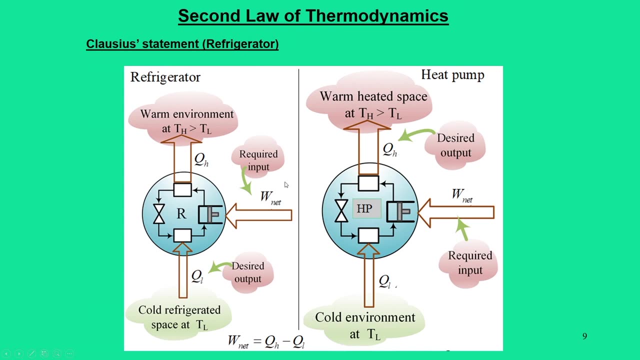 construct and heat engines that operates in a cycle and will produce no effect other than the extraction of heat from a reservoir to perform an equivalent amount of work. Now againthis, this second law of thermodynamics, can also be interpreted in another way, and we call this as a Clausius statements. So, in a Clausius statement, if you recall ourconcept. 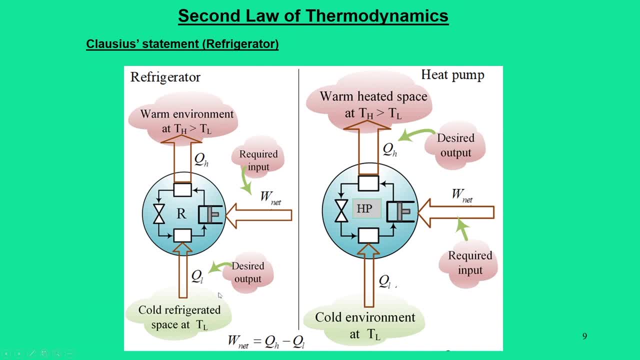 of refrigerators or heat pump, we say that the Q- L amount of heat is rejected from theis taken by the refrigerator or heat pump, from the low temperature sink, and it is rejected. and this, this refrigerator or heat pump, rejects q? h amount of heat to the heated space or warmer. 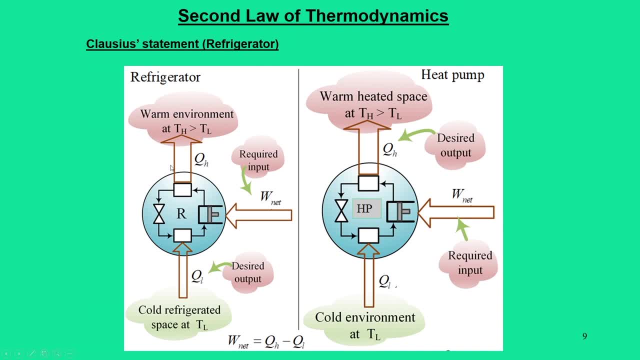 environment, So that to do this we must provide some that some of the network input into this cyclic device. So that is W net. Now, if you say this is the actual concept of run converting heat to work, or or taking heat from low temperature sink to the high, 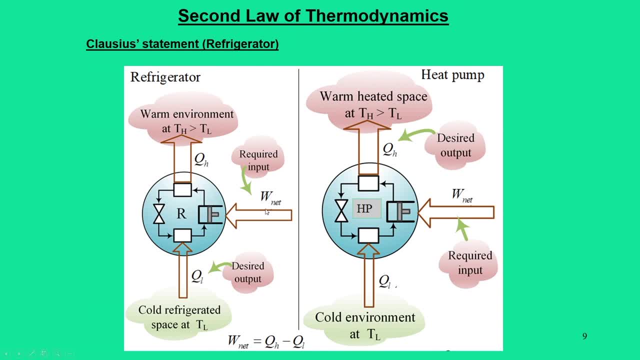 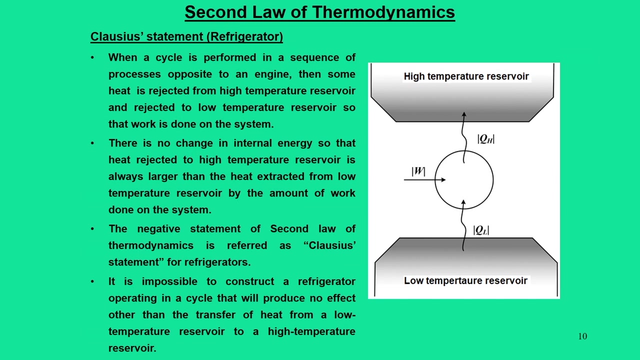 temperature source, which means that it must take some W net amount of heat to to perform this. That means to reject this q h amount of heat to the warm environment. So based on that, we all can also imagine in a similar way. what it says is that we have a refrigerator, or 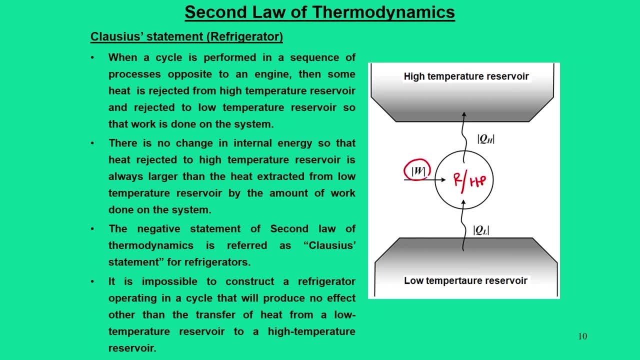 heat pump that takes W amount of heat and W amount of work input and while doing so, when it takes. So when it takes this W amount of work, then it can take q, l amount of heat from the low temperature reservoir and it can reject the q? h amount of heat to the high temperature. 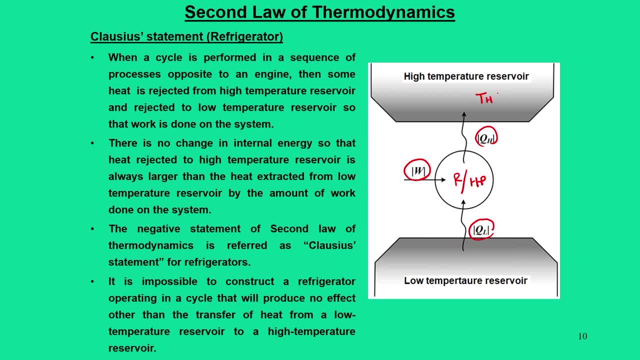 reservoirs. The high temperature reservoir is maintained at t h and low temperature reservoir is maintained at t l, And of course, in a similar sense, we can also view that process has to occur in a very quasi-static manner. Ok, Ok, and mostly it should be in isothermal process, so that the temperature of the reservoirs 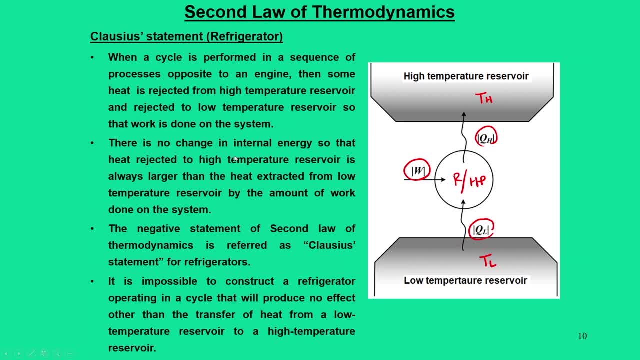 do not change And since there is no change in the internal energy, so that heat rejected to the high temperature reservoir is always larger than the heat extracted from the low temperature reservoir by an amount of work done on to the systems, So this frames the basics of the negative statement of second law, and that is commonly. 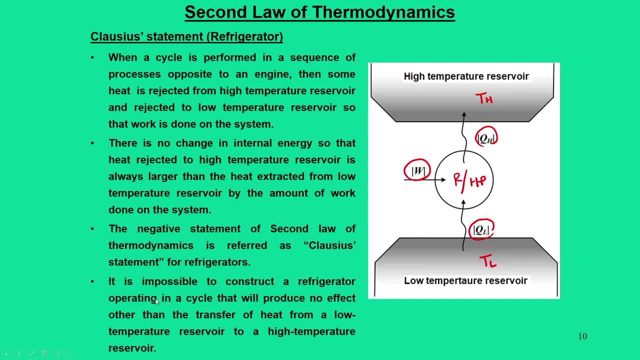 known as Clausius statement. So what it says is that it is impossible to construct a refrigerator that operates in a cycle and it will produce no effect other than the transfer of heat from the low temperature reservoir to a high temperature reservoir. I need to emphasize here the fact that the Kelvin, Planck and Clausius statements are 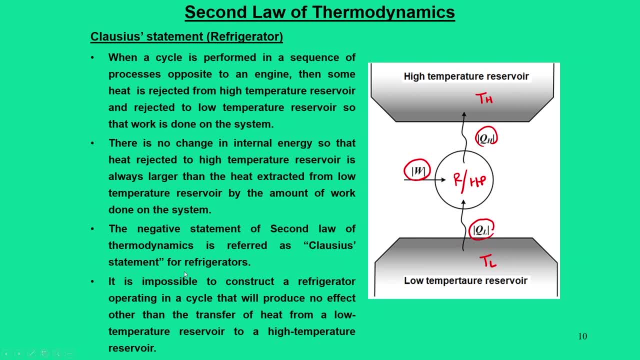 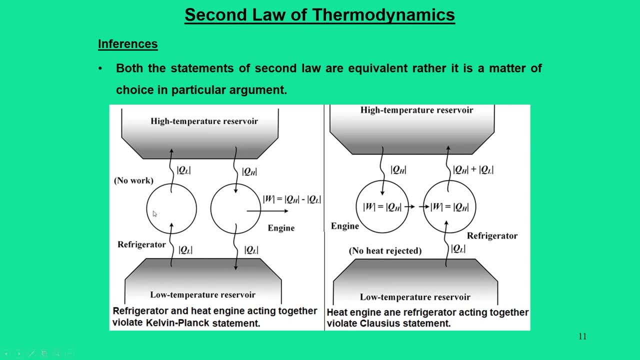 negative statements and they has to be written in this particular manner. So this is the second law and the third law And whatever may be the consequence, whatever may be the interpretations ofKelvin Planck or statement or Clausius statement of second law, one thing is ensured that both the both of them are the statements of second law and 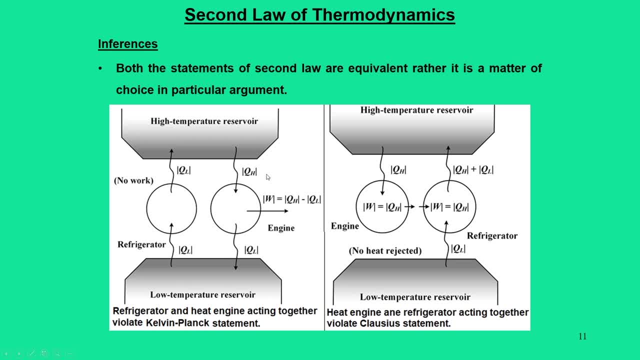 they are equivalent to each other. That means if some system violatesKelvin Planck statement, then it must also violate Clausius statements. And if some system violates Clausius statements, it also violates- should violate- Kelvin Planck statements. Here I have demonstrated the fact that how refrigerator and heat heat engine. 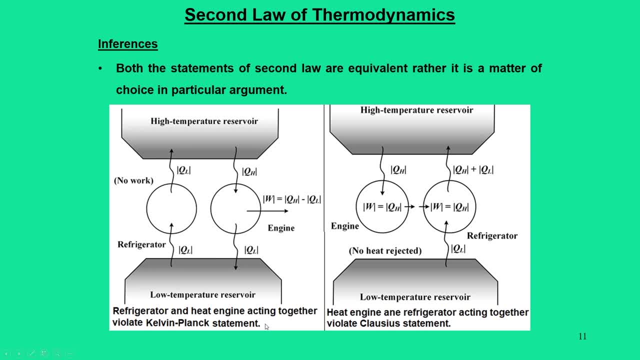 that acts together they violate the Kelvin Planck statements. What I can say here that we can initially view that thisR prior display of Kelvin State Arts on the lavender Rotterstock, The final LCB statement. we can stable unhealthy all Calvins State Arts myself. Now use this information and if it is not applicable before, 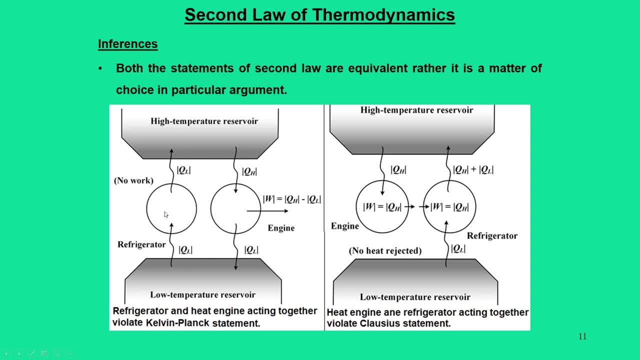 Andyou can say that, as ifthis, as if we can think about a refrigerator that takes Q L amount of heat and also it rejects Q L amount of heat to the high temperature reservoir, And in this process there is no work done in the systems. So this violates Clausius. 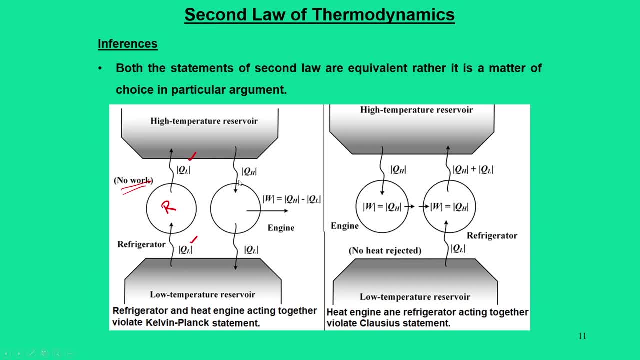 statements Now side by side. we can also construct another heat engines that takes, that takes Q H amount of heat and rejects Q L amount of heat. So in this process it it does the double amount of work, which is nothing but the difference. 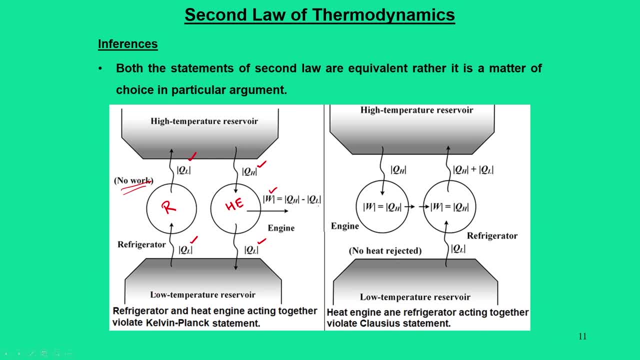 between Q, H and Q L. Now, if you take together both heat engine and refrigerator and they operate in this manner that it can be viewed that a system takes some Q, H and Q L Amount of heat and rejects and gives a W amount of work. butthat means this also. this will 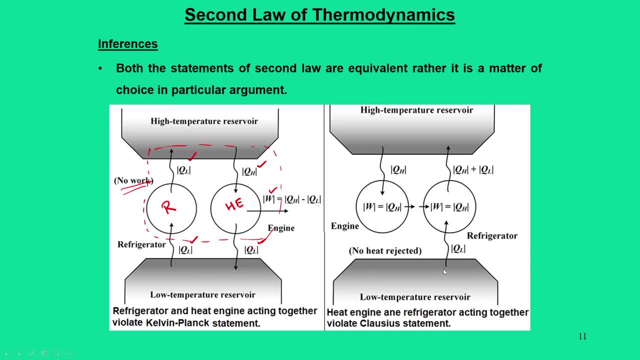 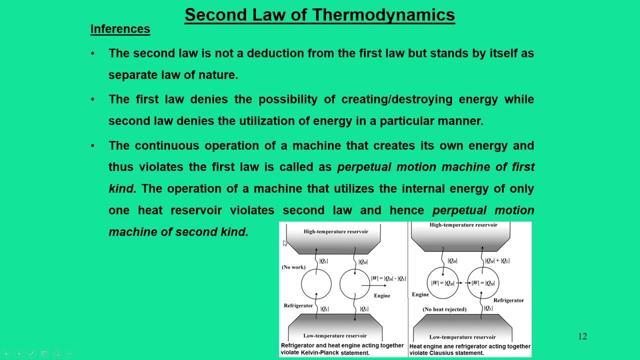 violate the Kelvin Planck statements. Similar logic also can be applied for a situations where heat engine and refrigerator. they act together and they violate Clausius statements. Now, after this, let me talk about some of the inferences that weday that that are given. 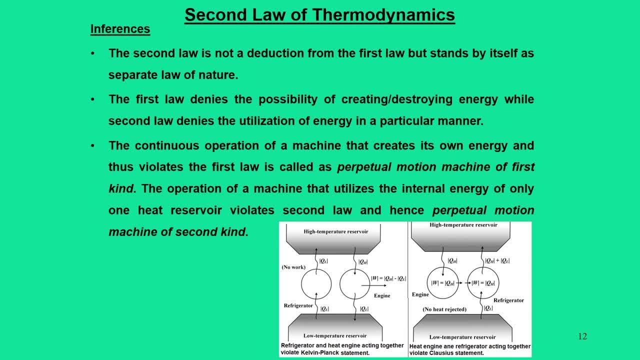 So let us look at some of the inferences that we that that are given. So let us look at some of the inferences that we that that are dealt from the second law of thermodynamics, So this second law of thermodynamics, a deductions. 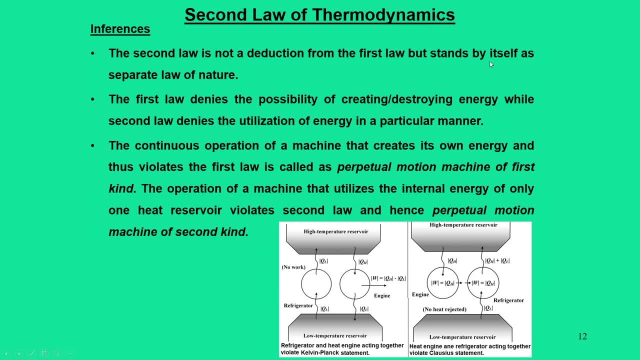 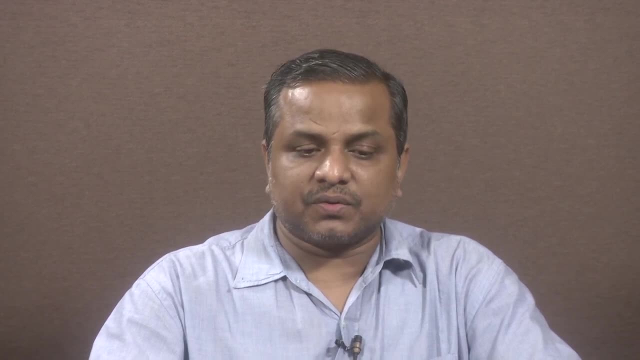 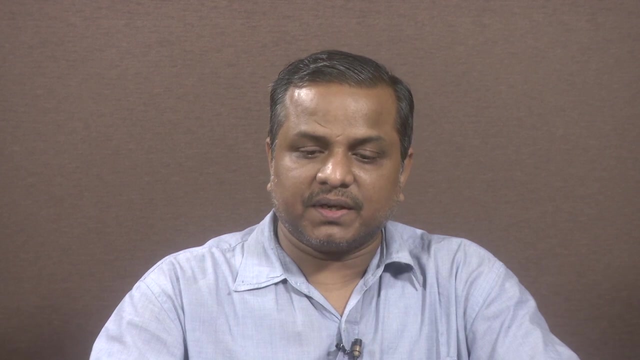 from the is not a deduction from the first law. rather it stands itself as a separate law of natures. So it puts the upper limit of any kind of devices that takes some amount of heat to convert into work. So it means all the heat cannot be converted to work completely. 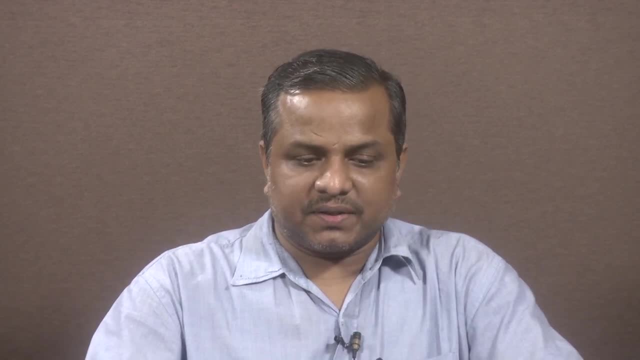 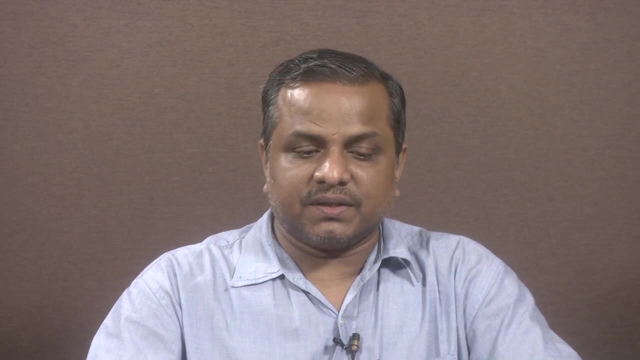 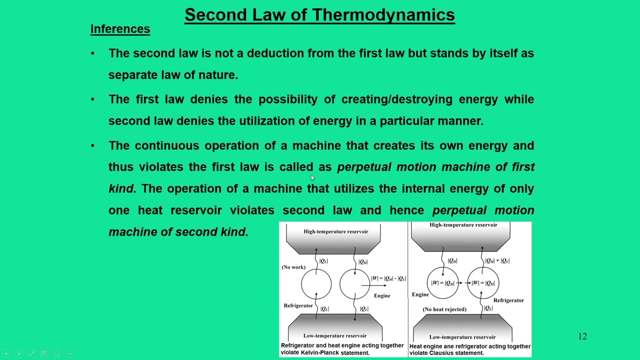 and indefinitely. And in a layman says we can say that the first law denies the possibility of creating and destroying the energy, while the second law denies the utilization of energy in a particular manner. So any device or machines that violates first law is known as perpetual motion machine of first kind. Any machine that violates 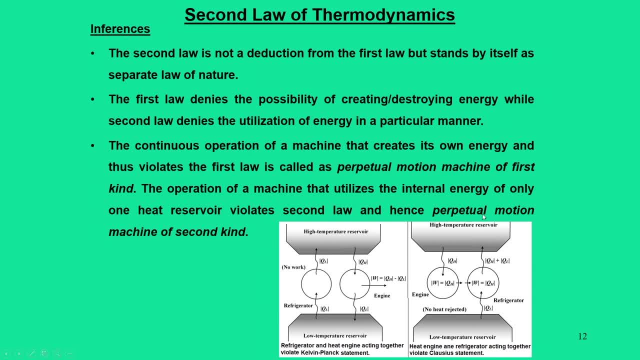 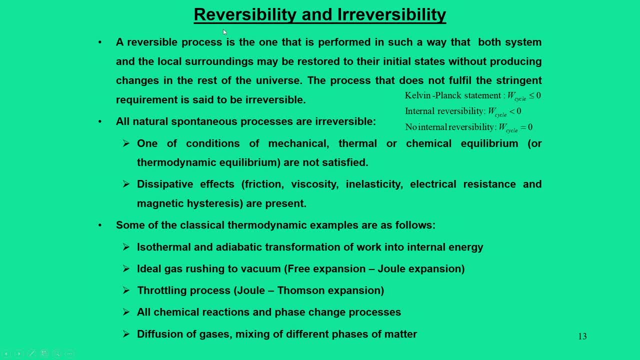 the second law of thermodynamics. We call this as a perpetual motion machine of second kind. Now we will go to the next segment, that is, reversibility and irreversibility. One thing we canderive from the Kelvin Planck statements that cyclic work is always less than or equal. 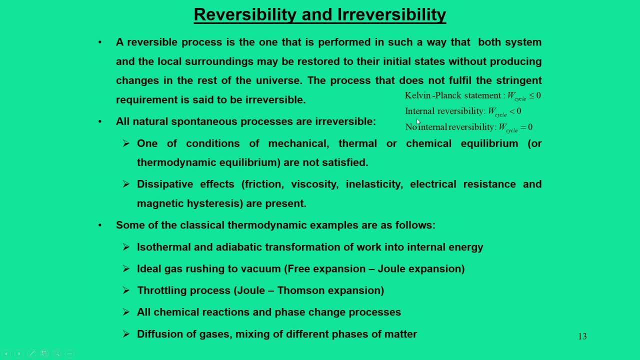 to 0. Now here there are. that are two possibilities in this equations. If you say that there is some internal hm hm Reversibility, there is some internal- sorry, internal- irreversibility, then the cyclic work is always less than 0. But if there is no internal irreversibility, the cycle 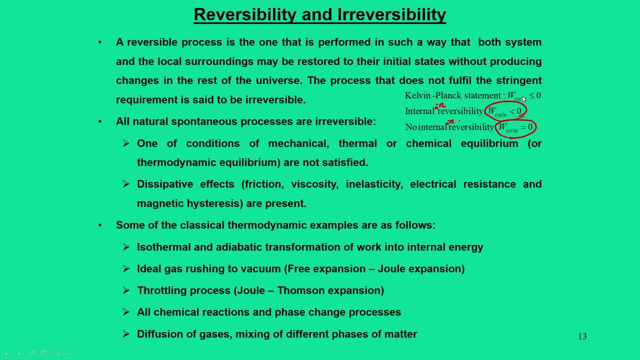 work is equal to 0. So this particular Kelvin Planck statement that cyclic work can either be less than equal to 0 or equal to 0 hm, It depends on the concept of reversibility and irreversibilities. So here we define this reversible process. 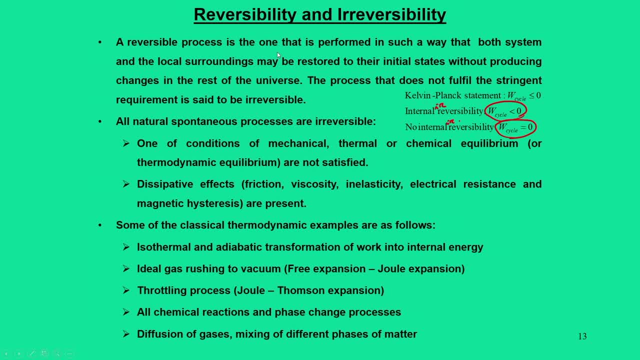 based on the second law in such a way thatone can view. this reversible process is to be performed in such a way that both system and local surroundings may be restored to the initial states without producing changes in the rest of the universe. This process does not fulfill. 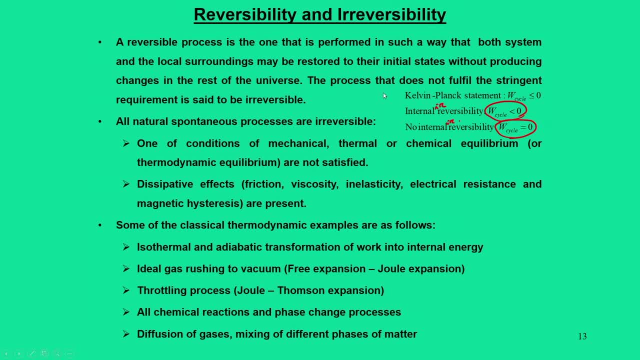 The requirement. and if the process is not, the process does not full this stringent requirement, then it is called as an irreversible process. Of course all natural, spontaneous processes are irreversible. One can say that when a process is not reversible, the conditions that has to be satisfied is that this it has to 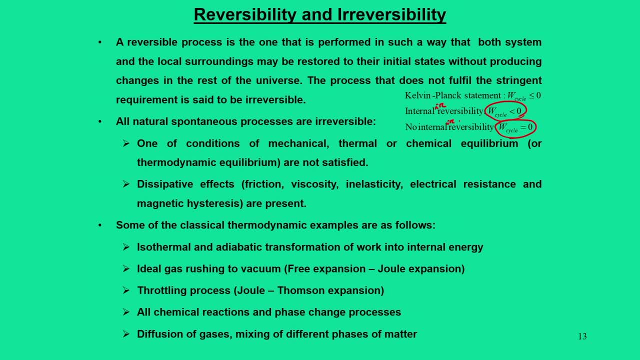 be in. this is the system and surroundings must be in the complete thermodynamic equilibrium. By thermodynamic equilibrium we mean that conditions of mechanical, thermal and chemical equilibrium is satisfied. Other option is that the, the, the irreversible. irreversibility is that there are some dissipative effects and which are not recoverable. So 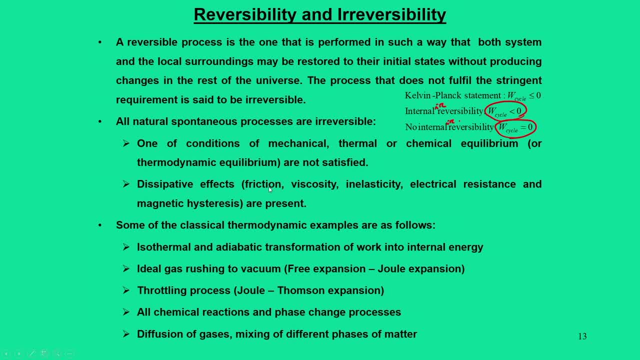 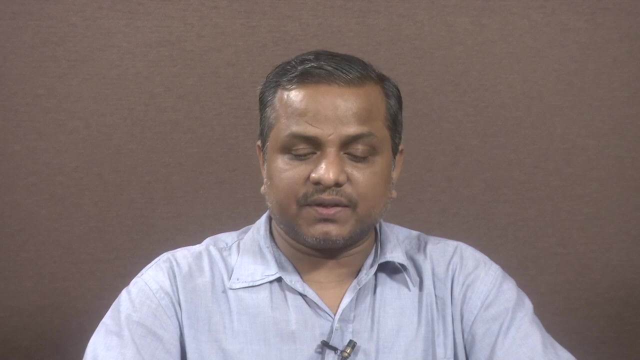 such Dissipative effects includefriction, viscosity, inelasticity, electric resistance, all other things. Now we are going to talk about some of the classical thermodynamic examples. that will talk about how the process is irreversible in nature. Some processes are like isothermal and adiabatic: transformation work to internal. 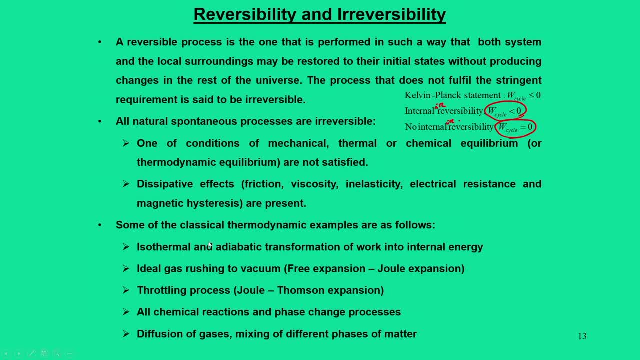 energy. So this is a procedure, So this is a situation where work is converted to internal energy. In one case process is isothermal, other case process is adiabatic. So in these processes we can say the, the, they are irreversible processes. And when ideal gas rosses to vacuum, that means as 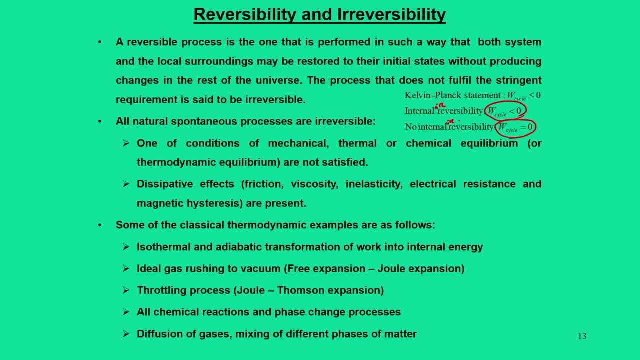 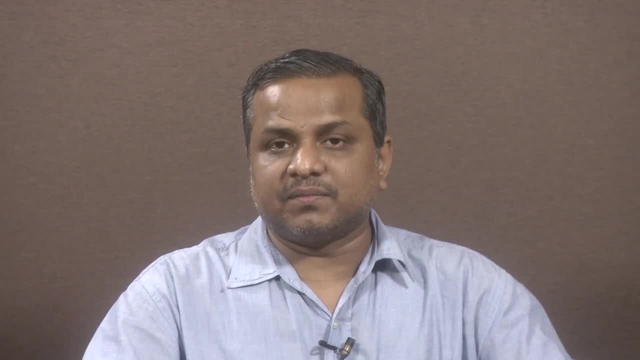 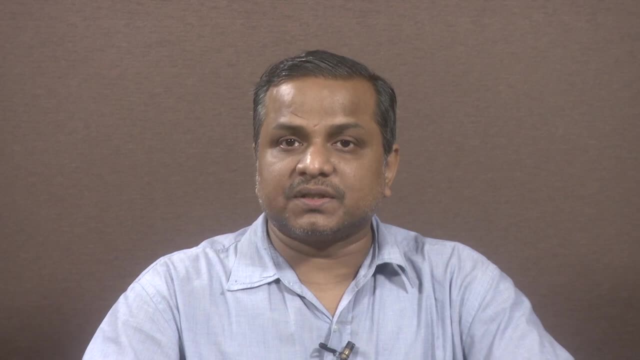 if you can imagine that there are two gases, they are separated by a completely, a vacuum. Ok, Complete partitions, and entire system isinsulated. and if you remove the partition, the gas which is at higher pressure will rush into the gas which is at low pressures. So this process, 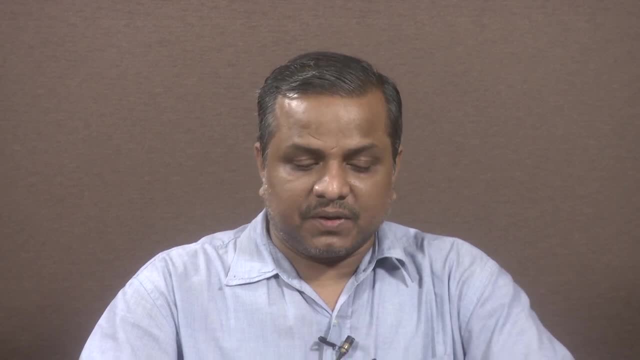 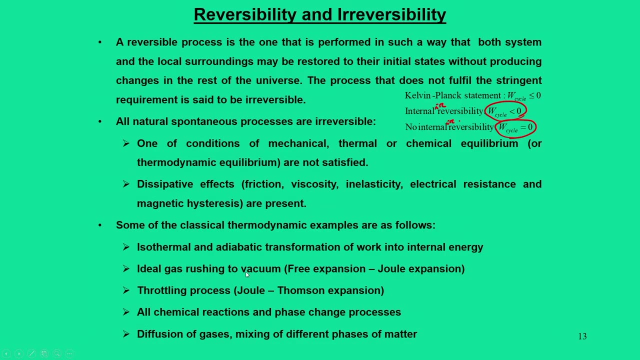 process we call as a free expansion process. ah, That means one can say that ideal gas. it is as if you can view this gas rushing to a vacuum. there is a tremendous pressure difference between them through a partitions, Other type of processes like throttling process, which is an irreversible process, all chemical reactions. 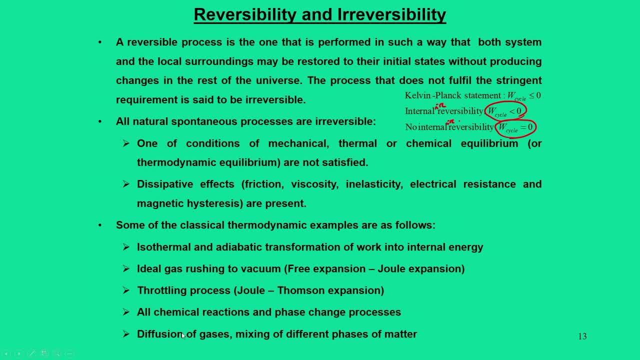 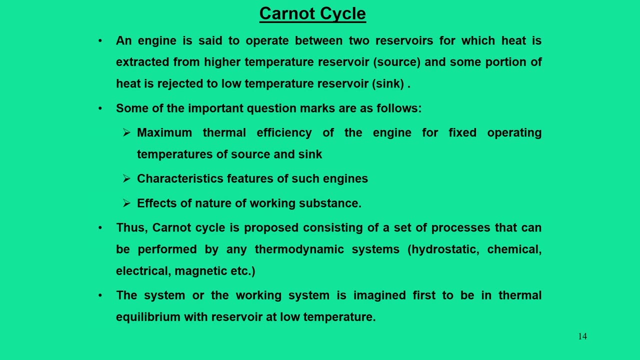 phase change process are consist are consider as a reversible process. diffusion of gases, mixing of different phases of matter are also consider as a irreversible process. Now, after complete understanding of reversible process and irreversible process, concept of work and heat, Now we are in a positions to define a heat injector. 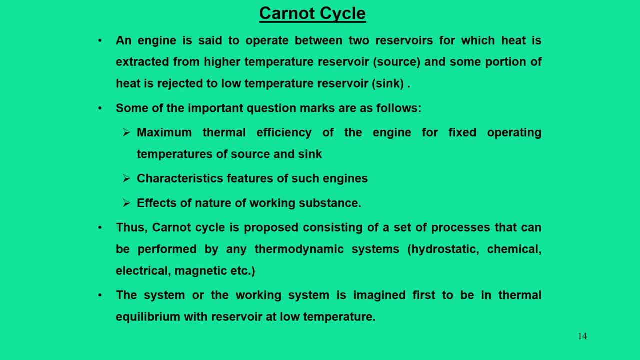 Ok, So that is also an essential component here. Now, this heat engineis based on the fundamental cycles and what we call is as a Carnot cycles. So this Carnot cycle, when it is introduced, to give the concept of engines, which means 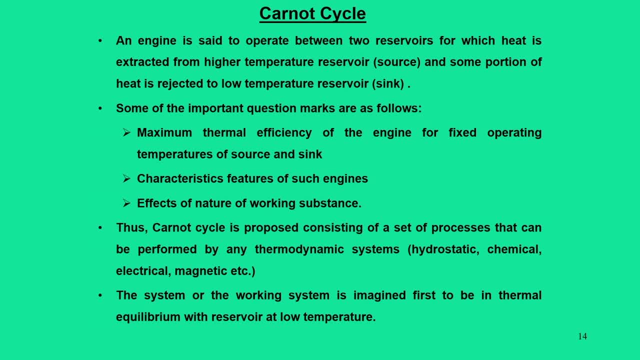 that the, the conversion of heat to work, has to be done through a device which is called as heat engines, And this conversion has to take place between two temperatures reservoirs: one at high temperature, which is called as source, other is at low temperature, which is the, which is the sink. But here the there are some important question. 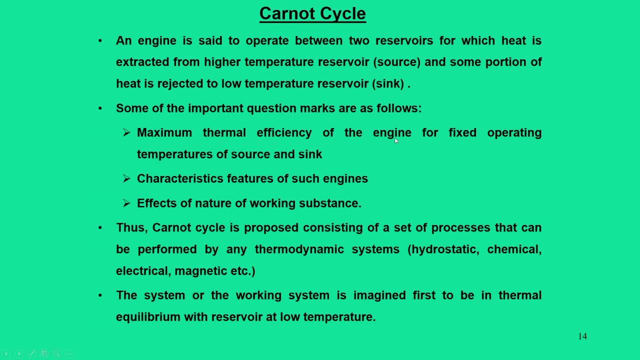 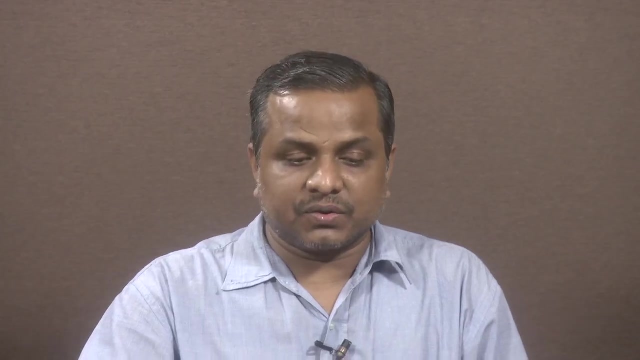 mark. that remains that what is the maximum thermal efficiency of the engines for a fixed operating temperatures between source and sink? what is the characteristics features of the engine? What is the effect of nature of working substance? because we say thatthere is a cyclic device, who takes the q, the heatwhich converts heat to work? So this questions needs to be answered. 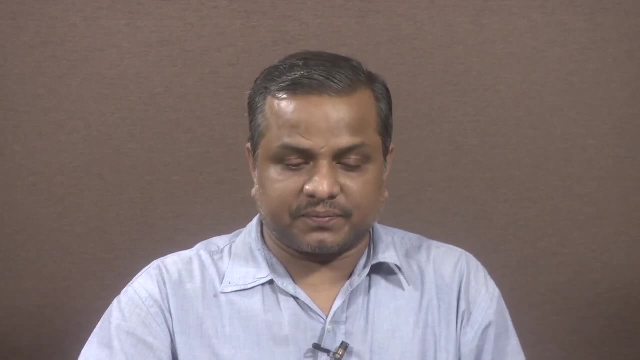 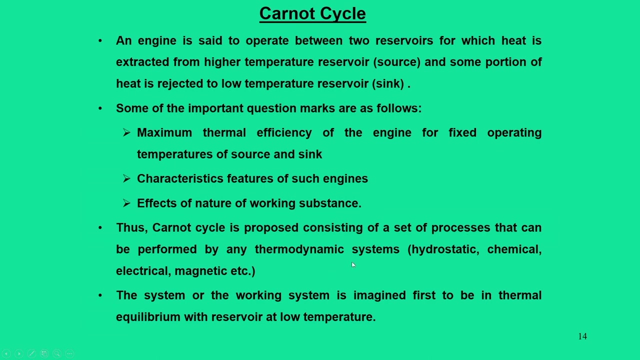 and this answer is possible by drawing a Carnot cycle. So a Carnot cycle is proposed, consisting of set of processes that are performed by the thermodynamic systems. By this we mean that it may. it is either a addressing Hydrostatic systems, chemical system, electrical systems and magnetic systems. The system: 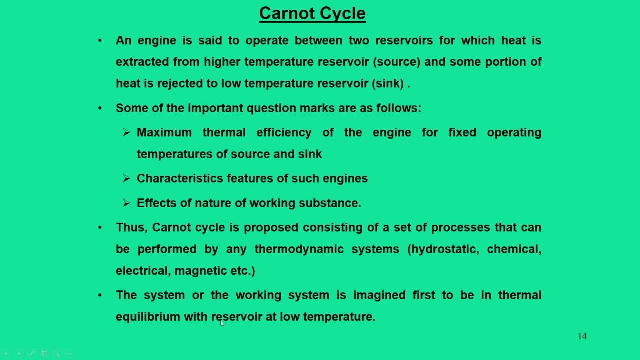 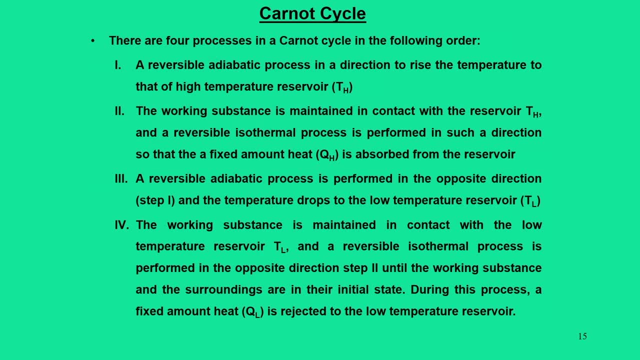 and the working medium is imagined to be the thermal equilibrium, with the reservoir at low temperatures. So this is the another assumption that we make. Now, when you say that a Carnot cycle, we say there are 4 processes that occur in the Carnot. 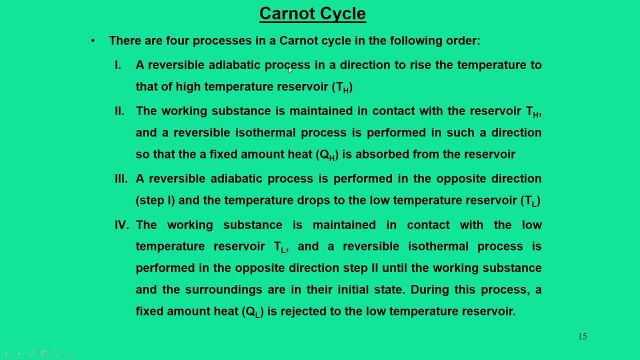 cycle. First one is a reversible adiabatic process that occurs in a directions to rise the temperature to high temperature reservoir. That means there is a reservoir which is at high temperatures and the process has to proceed in a directions to reach this temperature. T h The working. 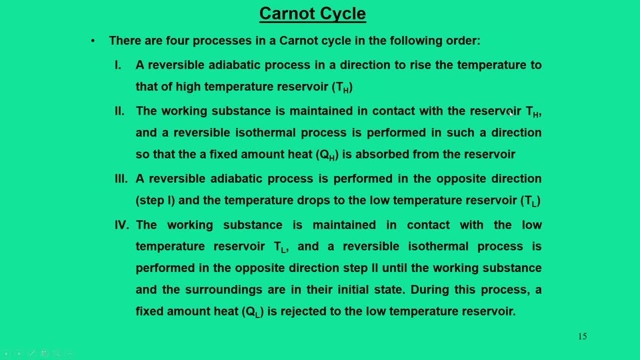 substance is maintained in contact with that reservoir T, h, and a reversible isothermal process is performed in a such a direction that fixed amount of heat- q, h- is observed from the reservoir. The third process is a reversible adiabatic process which is performed in the opposite. 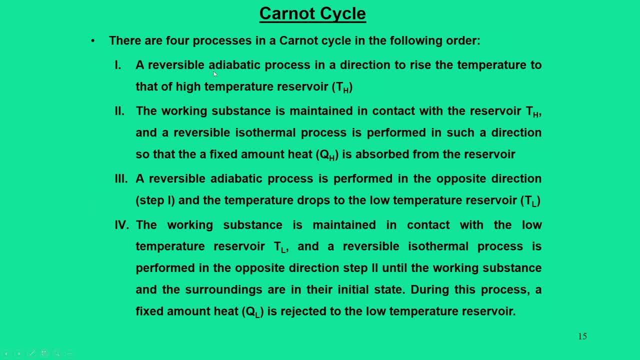 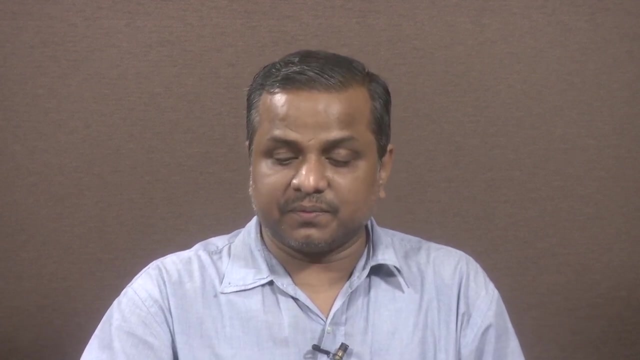 direction of step 1. that meanswherever. that means we should. this process should proceed towards the low temperature reservoir So that temperature drops, and the fourth process is the working substance is maintained in contact with the low temperature reservoir and the reversible isothermal process is performed in opposite direction of step 2 until the 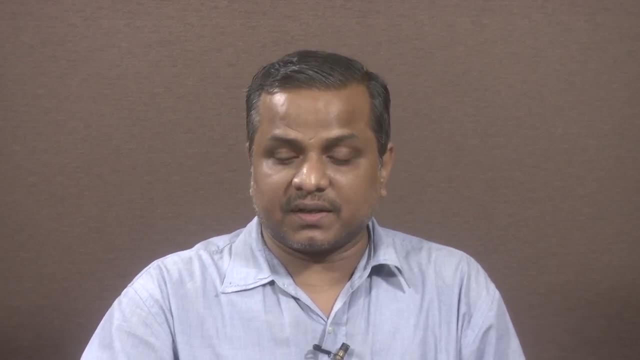 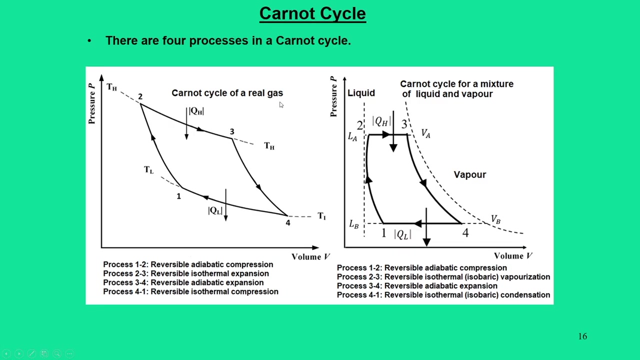 working substance and the surroundings are at the at their initial states. So during this process the fixed amount of heat, q l, is rejected to the low temperature reservoir. So these are the statement of all the four processes in a Carnot cycle. Now let us see. 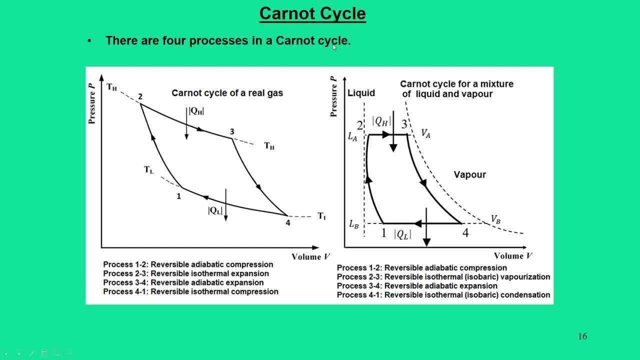 How these four processes are represented in a graphical form. Here there are two figures, which has shown here The first one. we say that Carnot cycle is drawn for a real gas. Sowhat we draw is that process 1- 2, which is a reversible adiabatic compression process. 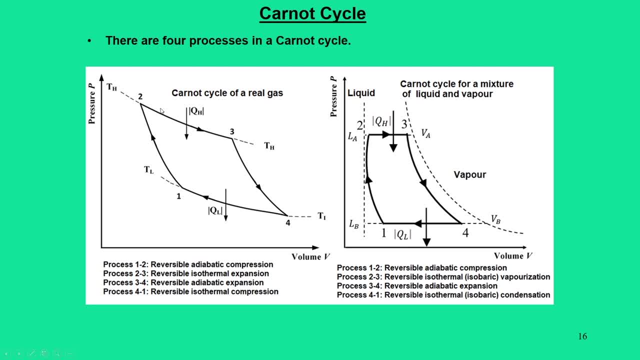 Process 2: 3 is reversible isothermal expansion, Process 3: 4 reversible adiabatic expansion and process 4: 1 reversible isothermal compressions. And of course all the processes are quasi static in natures. So this is done for a real gas. Now you can think about a cycle. 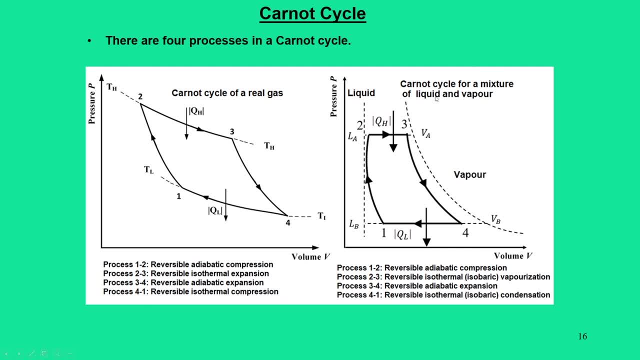 Carnot cycle, which is operated for a mixture of liquid and vapour. So when I say liquid and vapour, So it is about two limits. that meansLa and LB. that means we draw one vertical line: La and LB. So that means in this region, in this region, this state of the system is completely 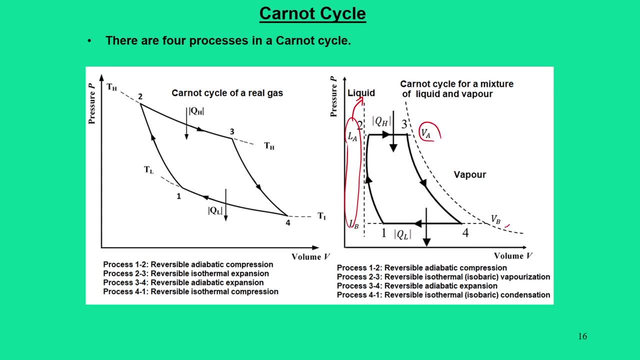 liquid and there is a region beyond Va and Vb. So in this region the state of the system is completely vapour and we are operating the Carnot cycle between these two lines and, infact, ah is nothing but the concept of Rankine cycle, wherewhere the cycle is operated between two. 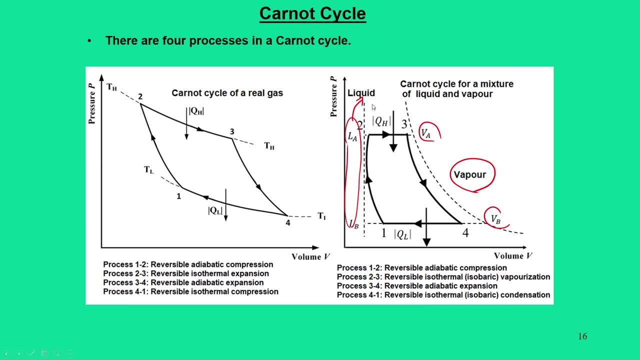 lines, liquid lines and saturated liquid line and saturated vapor line. So that is a different segment. but here, if you want to draw this, particular processes, what you call this, that process 1, 2 is a reversible adiabatic compression. 2, 2, 3 is a reversible isothermal and this 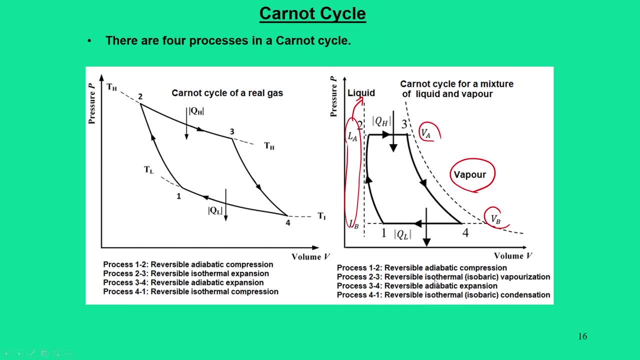 process. 2, 2, 3- since it is a phase change process, we say it is isothermal as well as isobaric process, and this process is known as vaporization Process. 3, 4 is a reversible adiabatic expansion. and then 4, 1 is again isothermal condensations. 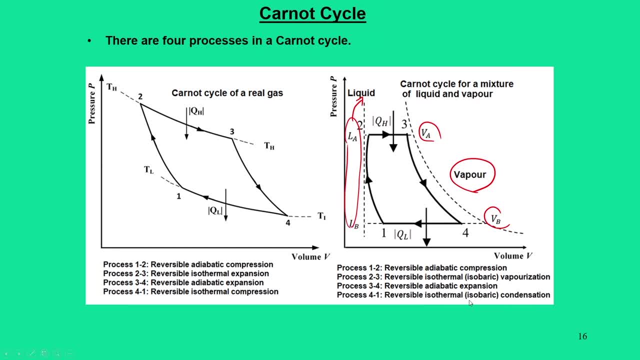 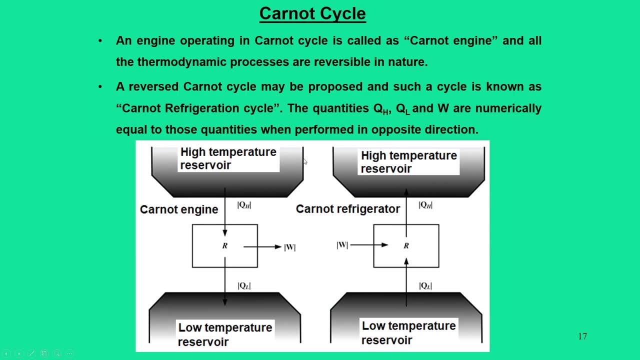 and this isothermal condensation process is also in isobaric nature, Because these two processes, that is, 2, 3 and 1, 4, 1, they occur at same temperature and pressure. ok, Thenhaving said this, now we are going to come back again to Carnot refrigerating. 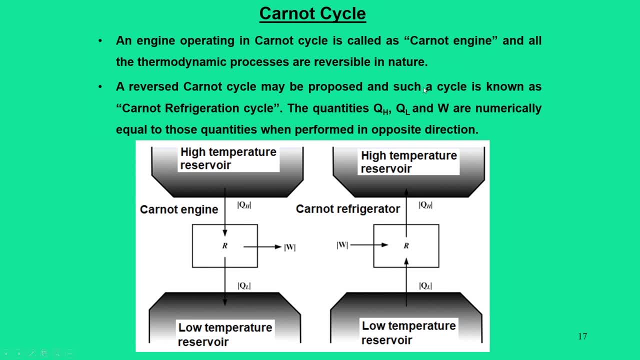 systems. that means how that similar concept of Carnot engine is going to be extended for a situations if it is a refrigerator. So when you say Carnot engines, it takes W, it produces W amount of heat, and we will say Carnot refrigerator, it takes W amount of heat to transfer heat from the low temperature. 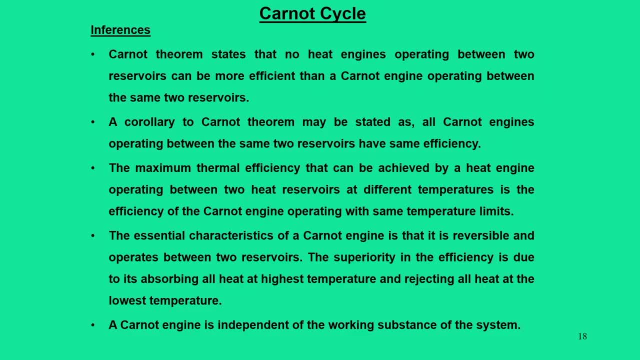 reservoir to high temperature reservoir. Now, from this entire Carnot cycle analysis we can frame some inferences. first one is Carnot theorem. It says that it states that no heat engines operating between two reservoirs can be more efficient than a Carnot engines operating between same two reservoirs. So we will 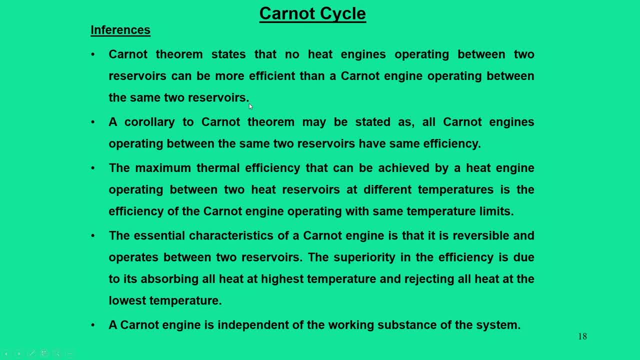 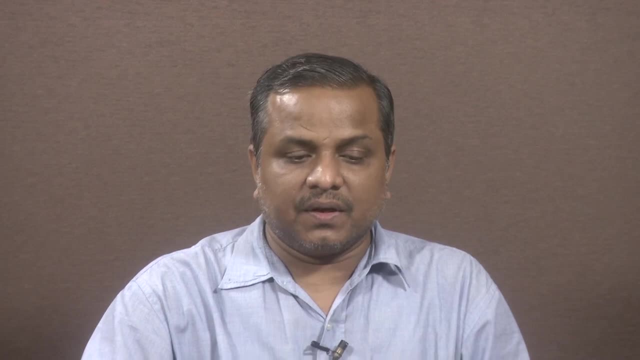 prove this, that what it means is that if a Carnot engine is operating between two reservoirs, that is, temperature, T h and T l, then any he other heat engines cannot have efficiency more than this Carnot engine. A corollary to this Carnot theorem is that all Carnot 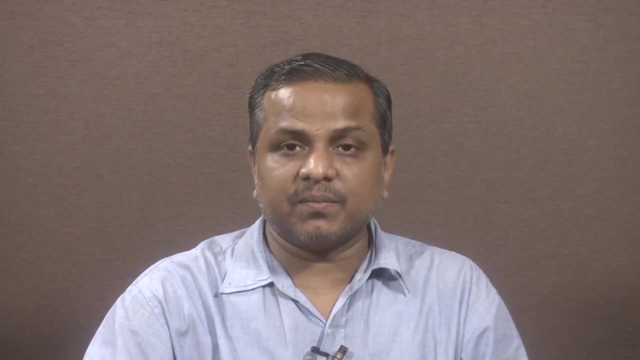 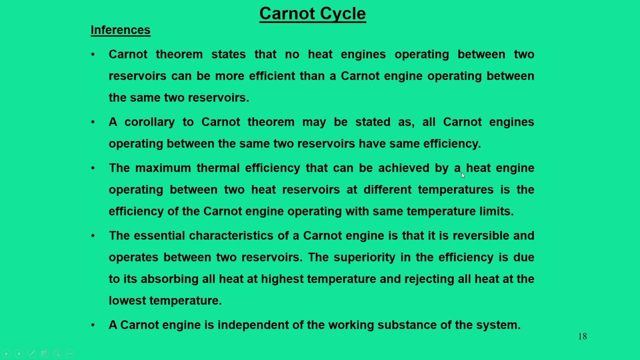 engines operating between two reservoirs have same efficiency. that is quite obvious. The maximum thermal efficiency that can be achieved by heat engine operating between two reservoirs at different temperatures. This is where this Carnot theorem is related. So if you temperatures, is the efficiency of the Carnot engines with same temperature limit. 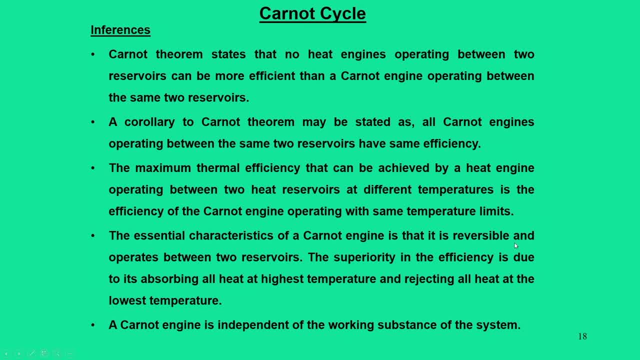 The essential characteristics of the Carnot engine is that it is reversible and operates between two reservoir. The superiority in the efficiency is mainly due to the fact it observes all the heat at higher temperatures. That means we imagine thisobservation of heat to occur in a very quasi static manner, or in this case it in isothermal manner. So 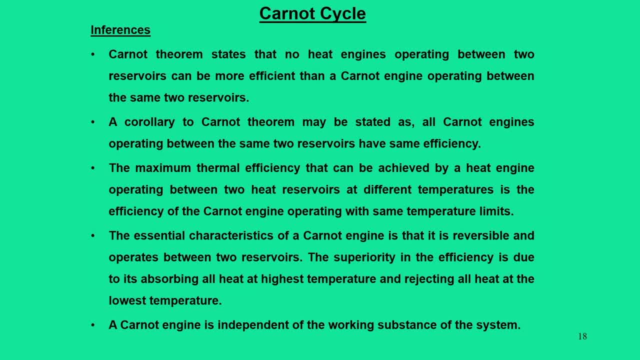 that temperature of the highest temperature of these things is does not change that may, and all the heat gets observed by the engine And it rejects also. in similar sense, it also rejects thatrejects all the heat at low temperatures And, moreover, we are subsequently, we are going. 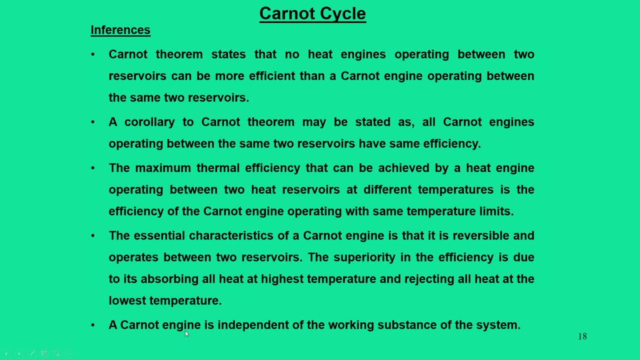 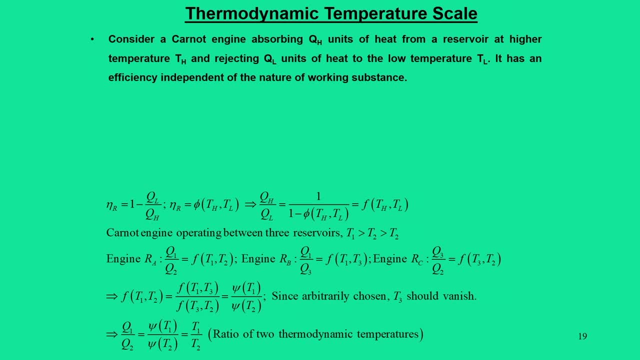 to say thatwe are going to prove that the Carnot engine is independent of working substance of the system. So now we will try to explain that. the Carnot worlds try to move to next segment and which is called as thermodynamic temperature scales. 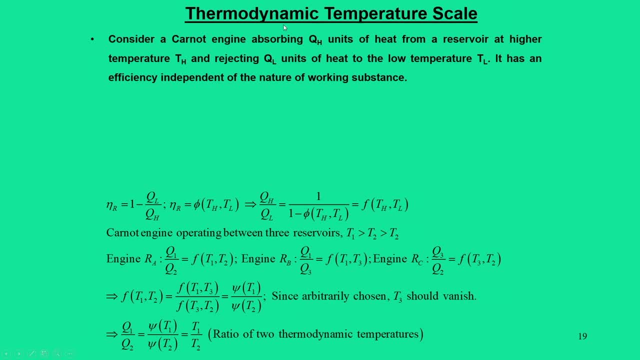 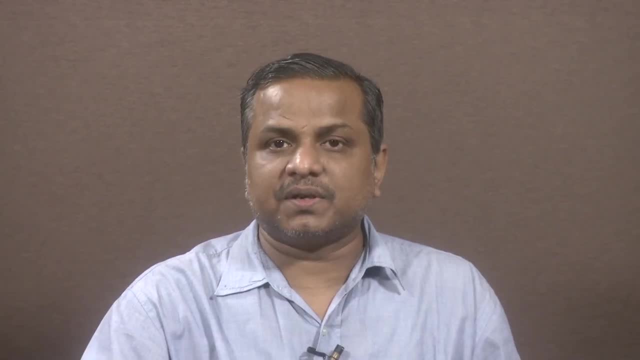 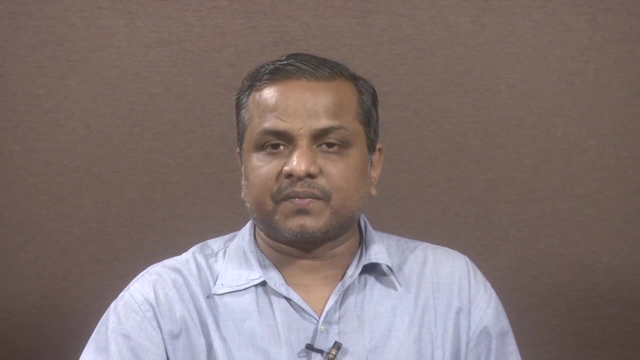 Now to prove these things. that means we always say that there is a high temperature reservoir, there is a low temperature reservoir and some heat is taken from high temperature reservoir and reject, rejected to low temperature reservoir. So so what is the correlation between this? 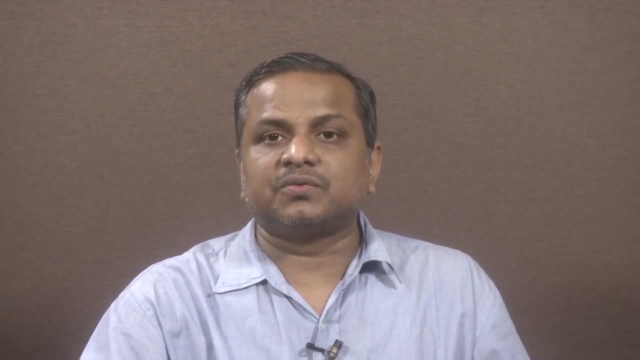 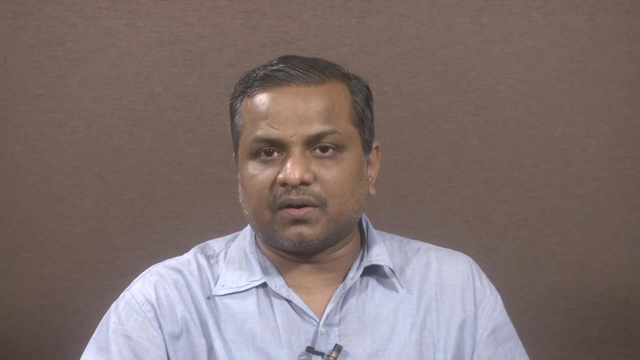 this heat and the temperature. So these are the calculations, So for this產i and the temperatures, and that too it is whether it is reservoir dependent or not, whether it is the working fluid substance dependent or not. So, to to bring this ambiguity, we are: 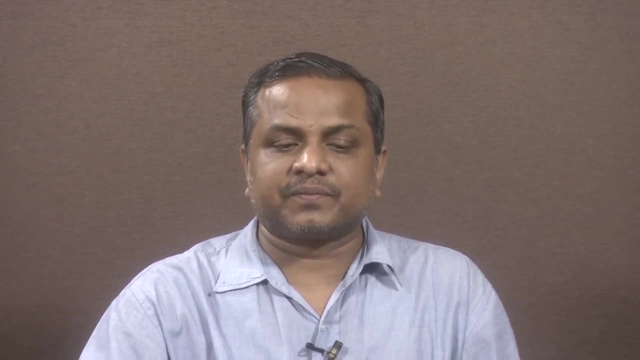 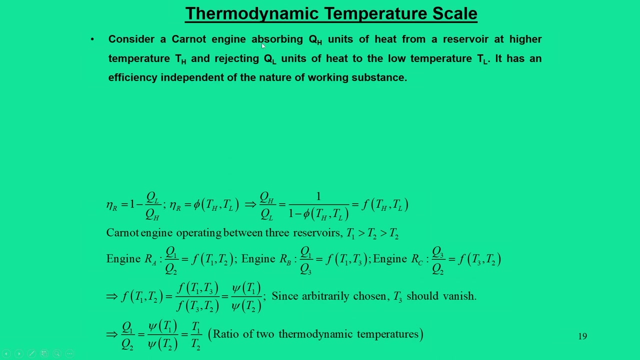 now going to define a scale and what we call as a thermodynamic temperature scales. So in to to prove this, we consider a Carnot engines that observes q- h amount of heat from a reservoir at temperature T, h and rejects q l unit of heat to the low temperature T. 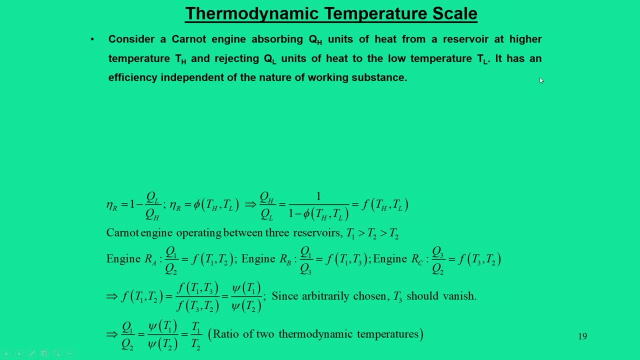 l and, of course, it has an efficiency which is independent of working substance. this you are going to prove. So, to consider this, let us view this particularexplanation in this manner, So we can say that we have a high temperature reservoir and which is maintained at T h and there is a low temperature reservoir. 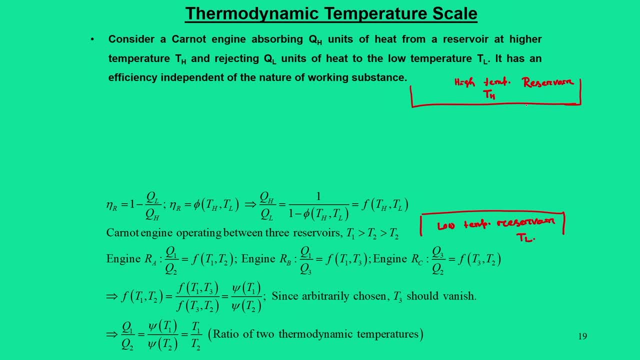 which is at T l. Now we imagine that one engine, which is nothing but a reversible engine, that is R a, which operates between T h and T l, and let us say it takes q 1 amount of heat and rejects q 2 amount of heat, and thereby it does W a amount of work. ok, 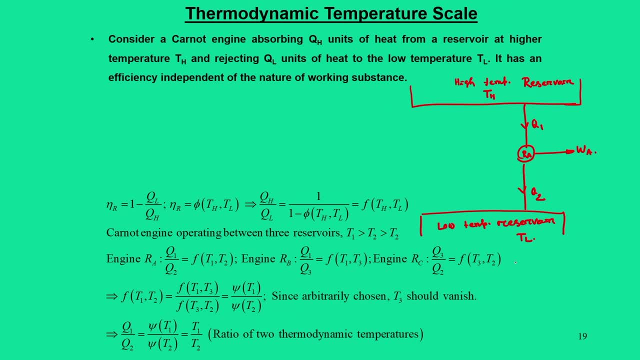 Now, within the samewithin the same temperature limit, we can also have a thermal temperature. So we can have another reservoir, T 3, and we can frame this, another heat engine which takes q 1 amount of heat and rejects, rejects q 3 amount of heat and thereby it does W b. 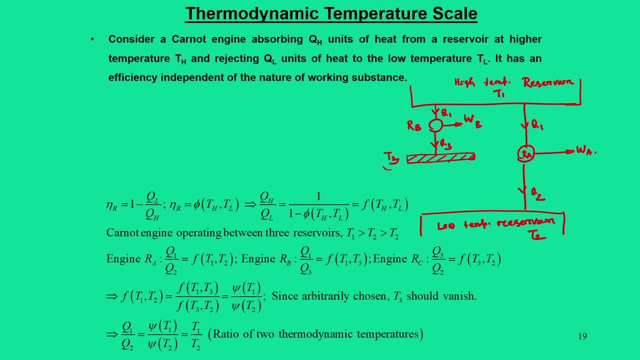 amount of work, imperial work. Now, between the reservoir T 3 and T 2, we can have another heat engine, reversible heat engine R c that delivers W c amount of work while taking Q 3 amount of heat and rejecting Q 2 amount of heat to the temperature T c. So if this is thethis is the explanation. 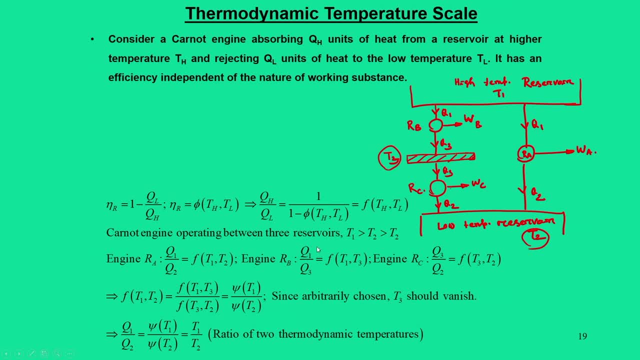 that we gave thatwe can. that means, in other words, we can say: there may be infinite number ofreversible engines that can be operated between the temperature T 1 and T 2.. So here we make a conditions, that for a three temperature reservoir T 1 and T 2.. 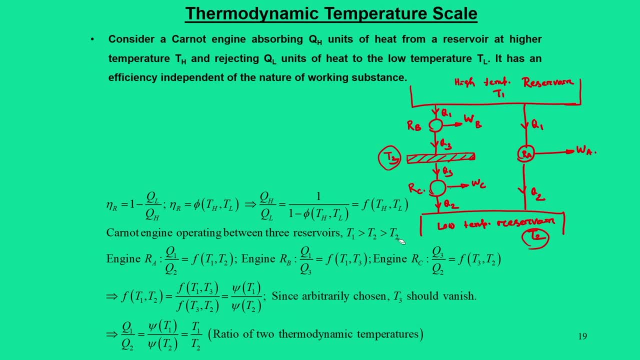 So T 1, T 2 and T 3, T 1 greater than T 3, greater than T 2. what we can write that for a reversible engines we can write efficiency of the reversible engine that is 1 minus Q L by Q h. So in other words we can represent this particular equations as efficiency in. 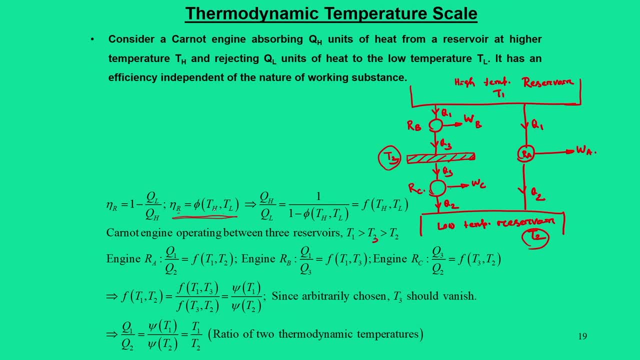 a functional form, Sothat is phi time, phi as a function of T h and T l. Now from this equation we can find another expressions, that is Q h by Q l as a function of T h by T l. So basically, 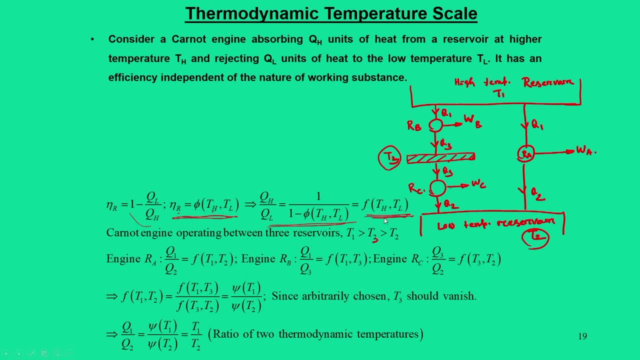 what you are writing, this particular equation in a functional form. So that means Q h by Q l in a function of T h by T l. Now here we will try to impose the situation that a Carnot engine operating between three reservoirs, T 1 greater than T 3 and T 4.. So that means 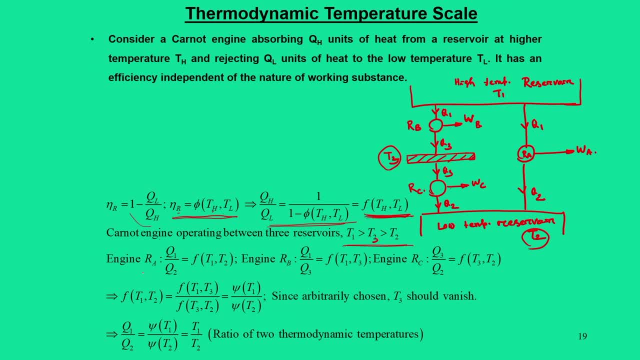 T 1 greater than T 3 greater than T 2. We can think that there is a engine, a R a, which of which is operating between T 1 and T 2.. So we can write Q 1 by Q 2 is a function. 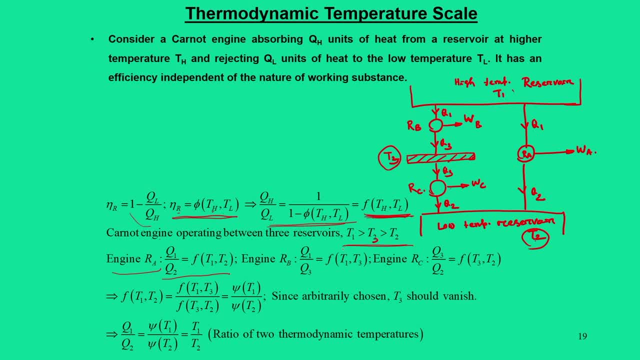 of f, T 1 and T 2, Another engine that operates between T 1 and T 3.. So Q 1 by Q 3 is a function of T 1 and T 3 For engine c. this Q 3 by Q 2 is a function of T 3 by T 3, So we can. 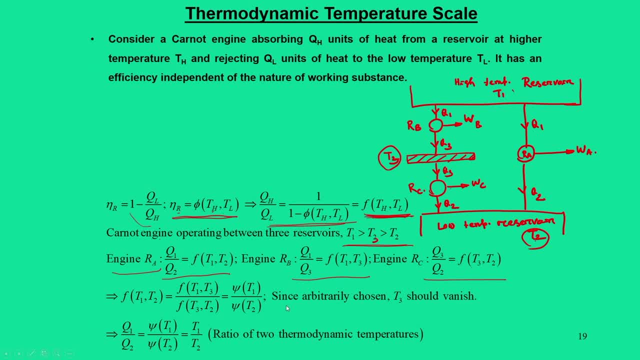 take this ratio, what it turns out to be is that the functional form f- T 1 and T 2 is equal to f- T f, T 1, T 3 and f- T 3- T 2. So here the you can see thatwe have a equations. 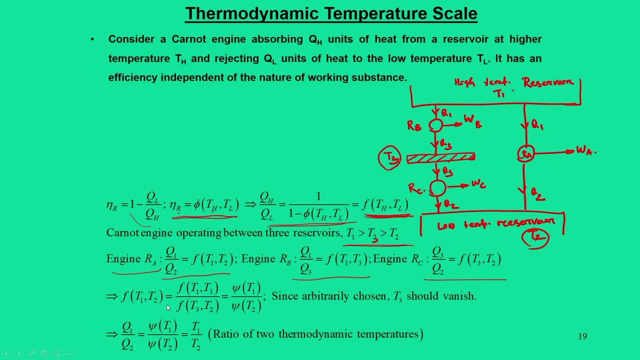 and in the left hand of side of the equation there is no term T 3, but where the right hand side term, that is, there is a function, there is a term T 3. So we can think that these relations exist in a such a way that the T 3 vanishes, while 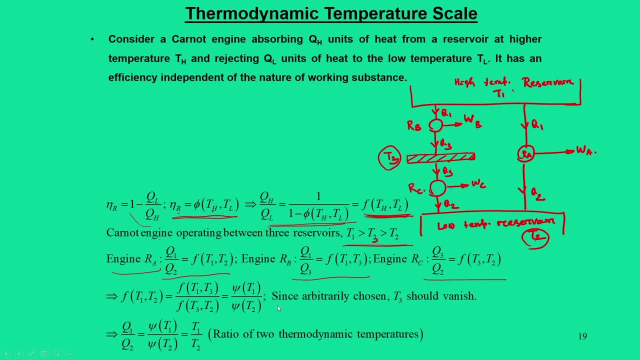 taking this ratio, And so that meanssince, since this, this functional relations are arbitrary chosen, So T 3 should vanish, So in, in other words, we can write: f, T 1and T 2 is a nothing but the ratio of some other functions, functions psi, T 3. 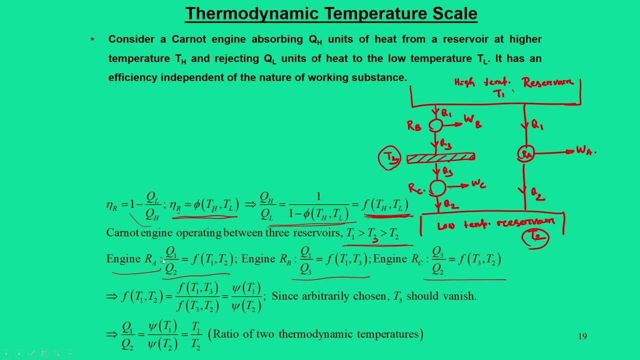 So by this concept we can now write this particular equation in this manner, where it say: Q 1 by Q 2 is a is equal to psi T 1 divided by psi T 2, And hereif youchoose the, choose the functional relation in such a way that simplest one would be a linear relations. So 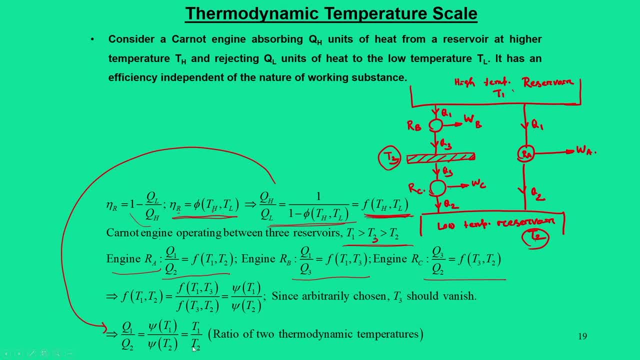 So, if I can say that we choose this, the relation, in such a way that the ratiowill choose in which we should be, the ratio Q 1 by Q 2 should be equal to the T 1 by T 2, and such a situation. 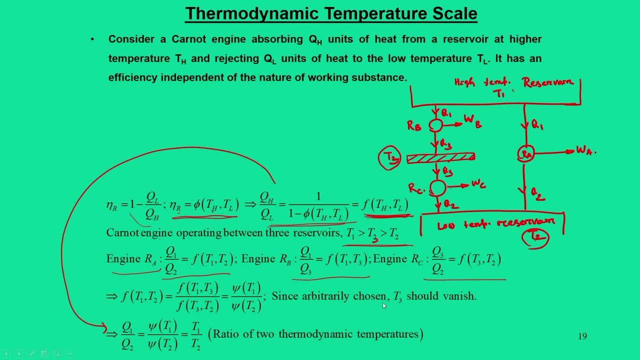 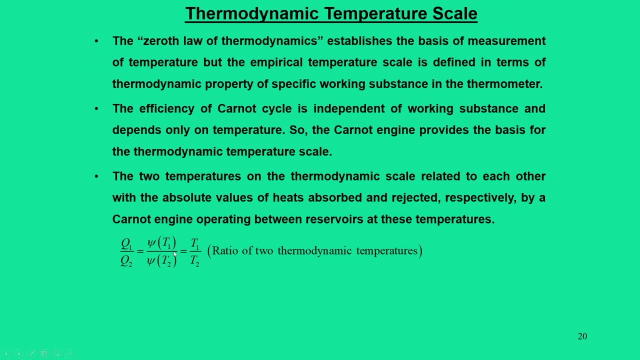 we call this as a ratio of thermodynamic temperatures. Now let us see what is its significance. Now, when we say this- Q 1 by Q 2 as a function of T 1 by T 2, it means that we are now correlated, that we have temperature T 1 and there is 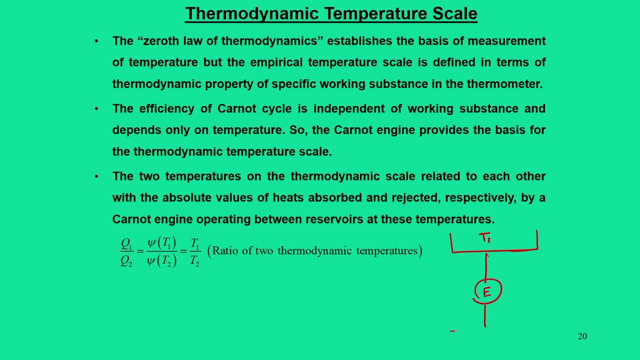 a engine. there is a low temperature, T 2.. So it is a source and it is sink and it is low and we have Q 1 amount of heat and it is goes as Q 2 amount of heat. by virtue of this work that is going out as W Now. we have now framed this equation: Q 1 and Q 2. 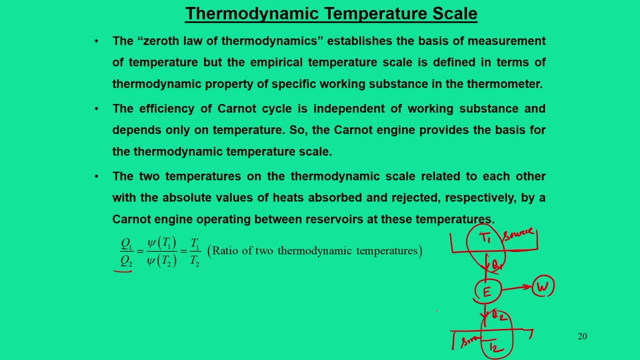 this ratio and Q 2 by T 2. this ratio and this functional relations becomes a linear relations, that is, T 1 by T 2, with certain conditions, and that conditions we are going to establish such a way that the one of the important relation will remain, that it has to be Q 1 by Q 2 is 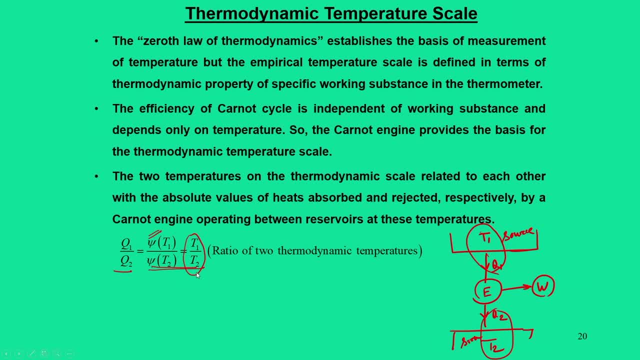 equal to T 1 by T 2.. Now, under what circumstances this relation is valid? So this, we are going to prove. So for that, what has been? So, what has been ah, chosen is that we take some kind of temperatures and this temperature has to be a T 2, we can. 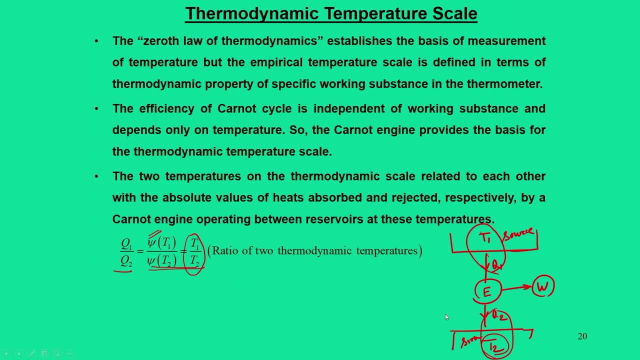 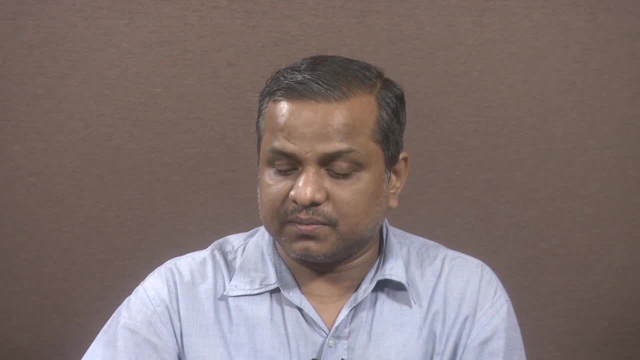 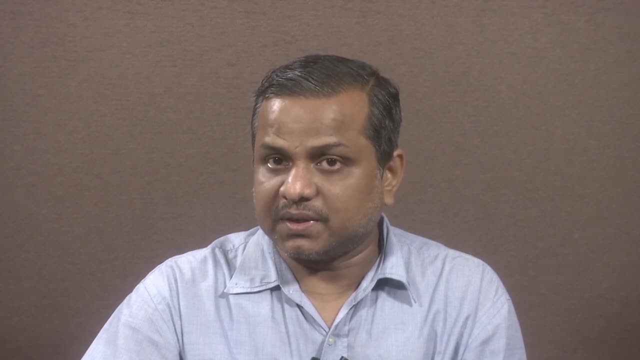 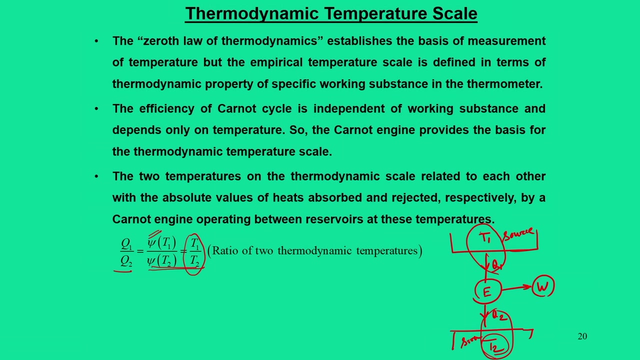 bring it to a temperature which is nothing but the triple point of water, for which we know what is the value of heat transfer, that isduring when the heat is rejected to at a temperature which is nothing but the triple point of water. So, that point of time, what is the amount of Q? So this will give you the basic definition. 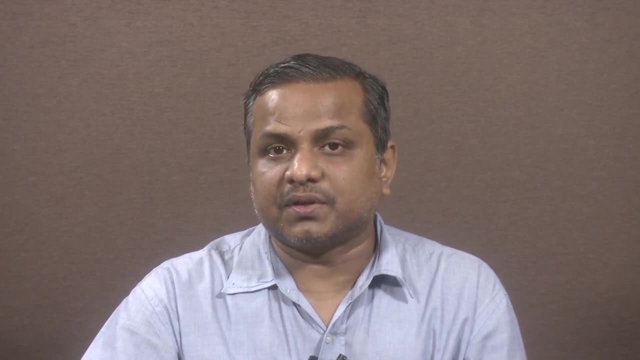 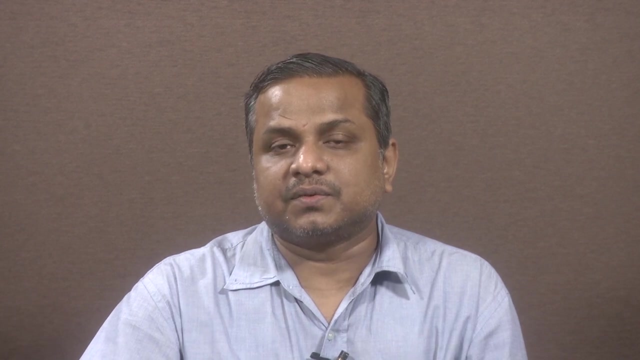 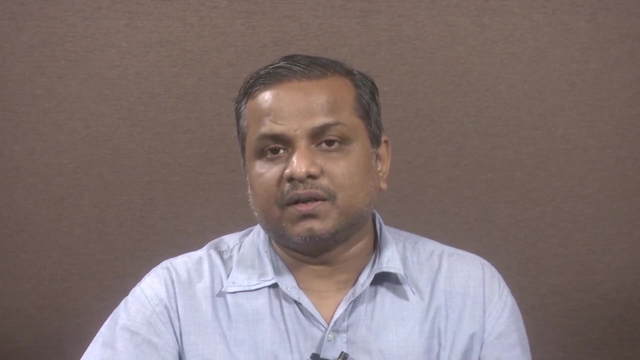 of another temperature for the, which is called at absolute temperatures. At that absolute temperatures, when you say triple point of water, there it is. we can say that all the three matters coexist. That means if you, if you take a water at, may be 273 Kelvin. 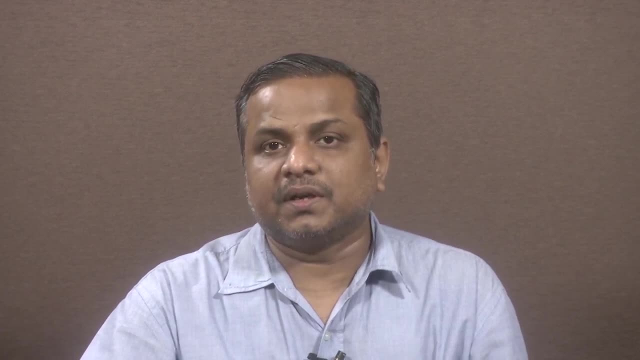 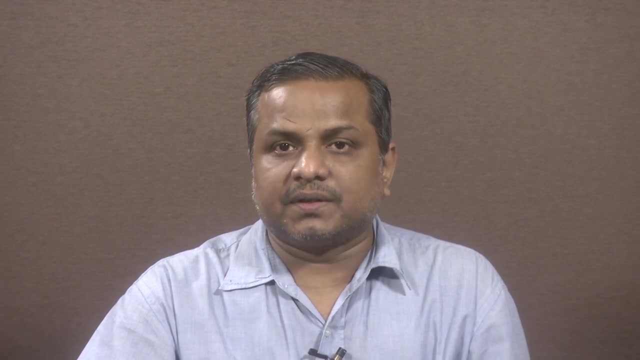 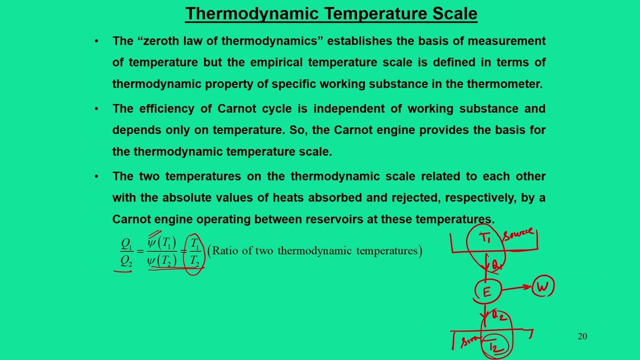 we can say that Solid, liquid and vapour, all the three phase, coexist. At that point the choice of working substance becomes now independence. So this is the essential concept of definition of an absolute scale. So if you try to correlate with what temperature? 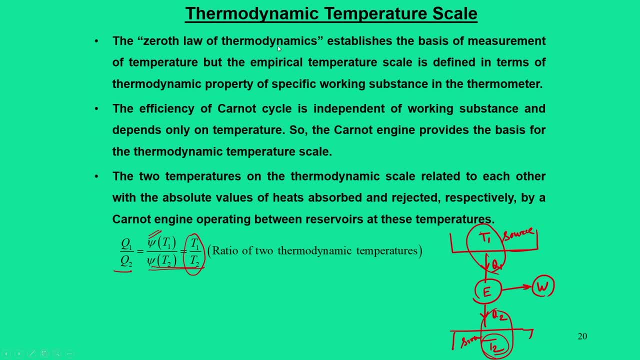 what we have studied. while talking about zeroth law of thermodynamics, we said that There is a temperature scale which depends on the specific working substance, For example, when you say gas thermometer, when you say mercury thermometer, so all these things are. 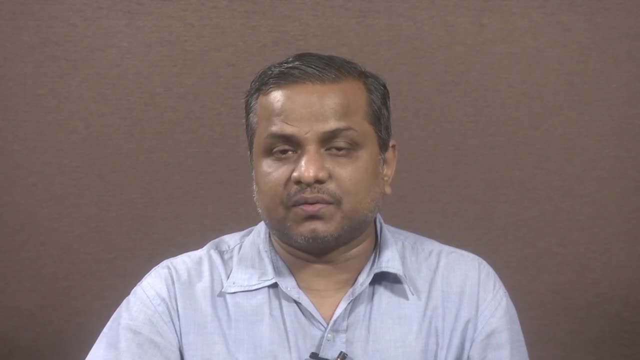 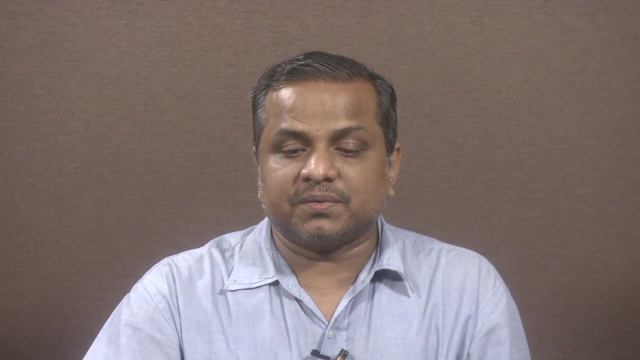 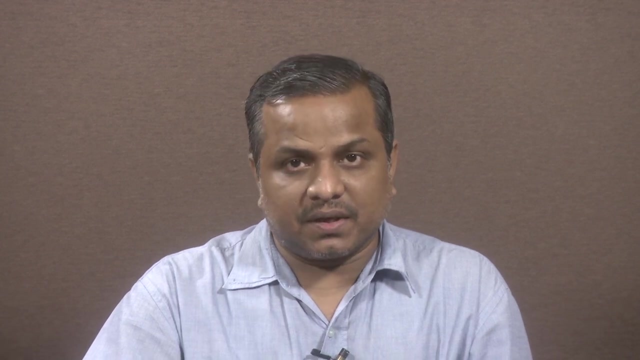 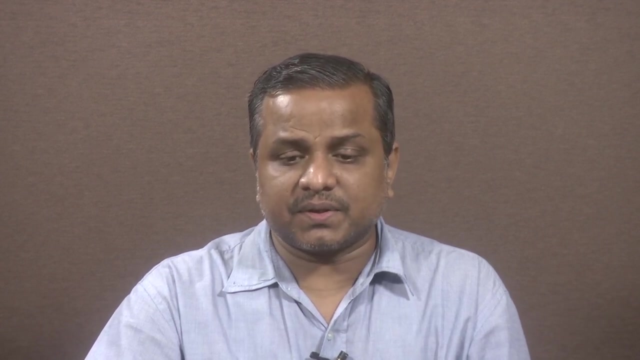 essentially dependent on the working substance, whether it is a mercury or it is a gas or any other substance. So so, zeroth law of thermo thermodynamics. when it gives the concept of temperature, it always relates with the nature of the working substance. But here, when you deal with the Carnot cycle and the thermodynamic temperature, 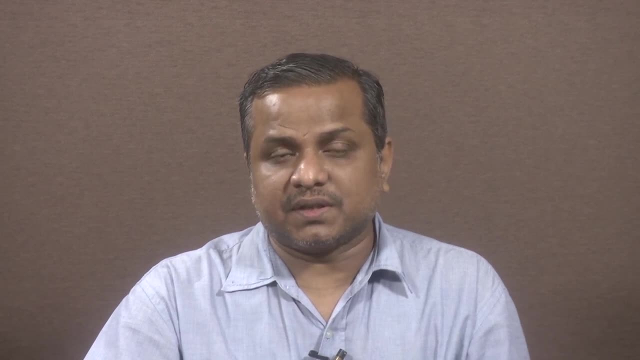 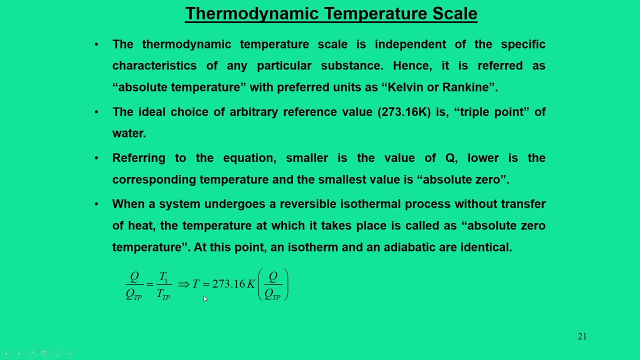 scale. we are going to choose a temperature scale in such a way that relation between q 1 and q 2 are linear. at the same time, the choice of working substance is independent. And for under such circumstances, we say thatwe write this q 1 by q 2 relations in a form. 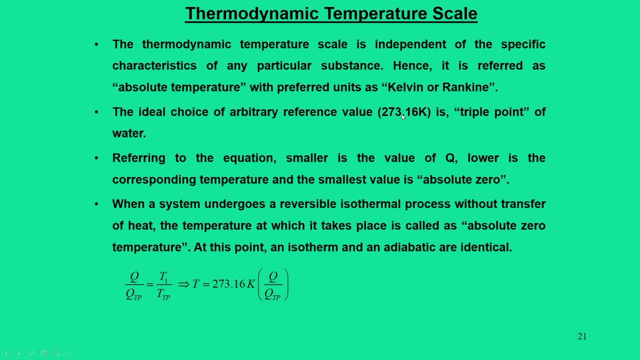 that if you take the triple point of water, which is nothing but 273.16 Kelvin, where the choice of working substance become independent, that point T becomes 273.16 q by q T p. And this now in this equations, if q is equal to 273.16 q by q T p, 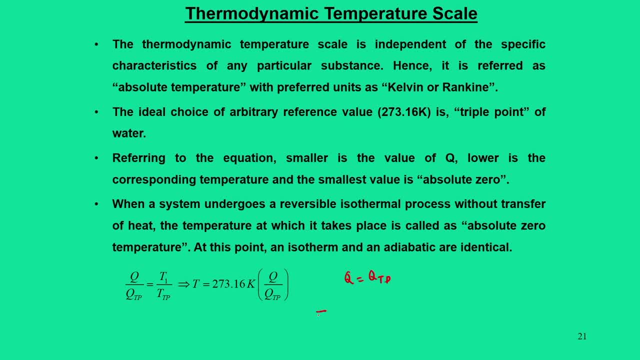 And this now in this equations: if q is equal to 273.16 q by q T p, And this now in this equations: if q is equal to 273.16 q by q T p, then this will imply T is equal to 273.16 Kelvin, and this is nothing but your absolute. 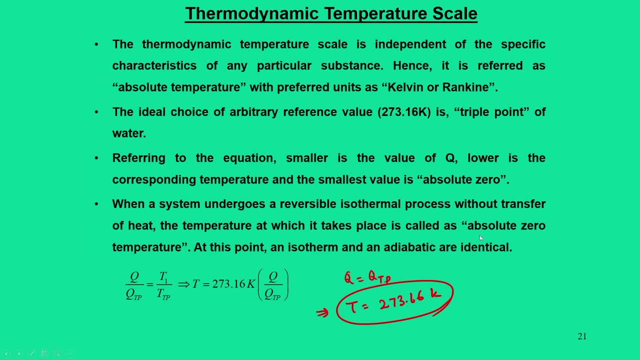 temperatures. So definition of absolute temperature can be written like this: and this definition we get it from the Carnot theorem, from the from the Carnot cycle informations. So what does it say? that when a system undergoes a reversible isothermal process without transfer of heat, then the temperature at which it takes place. 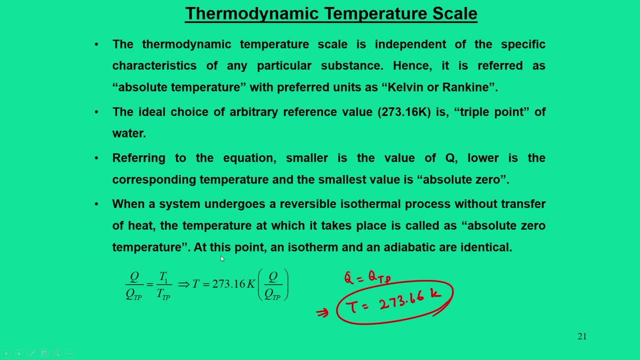 is called as absolute temperature. Now, at this point, the there is no concept of isothermal or adiabatics. all are identical, And herethe choice of unit, which can be either Kelvin or Rankine. So many times like we the standard practice that we are using. 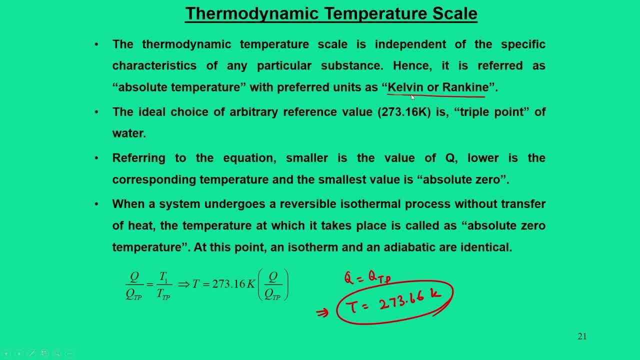 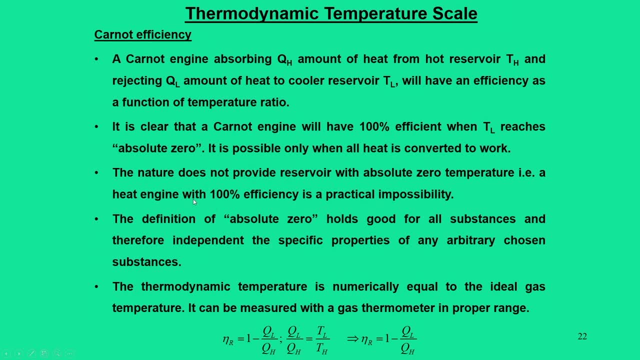 SI system of unit, and that is, that is, Kelvin, and if you go for theBritish systems, it is referred as Rankine. Now, at this particular point, we are now able to define an efficiency, what is called as Carnot efficiency. So theif you look at this particular equation, 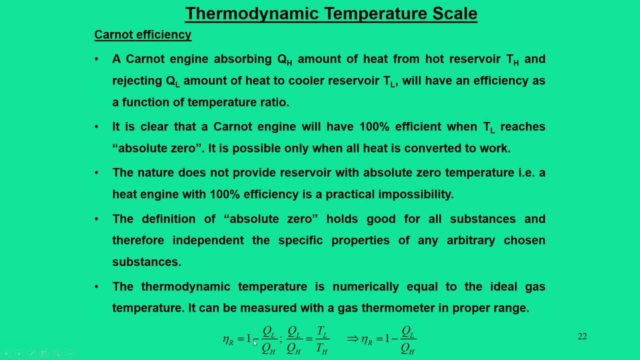 again that for a reversible heat engines we can write this expression of efficiency as 1 minus Q L by Q H. Now putting Q L and Q H is equal to T L by T H. we can write: for a reversible engine: this efficiency comesas a ratio ofsorry1 minus T L by T H, And here: 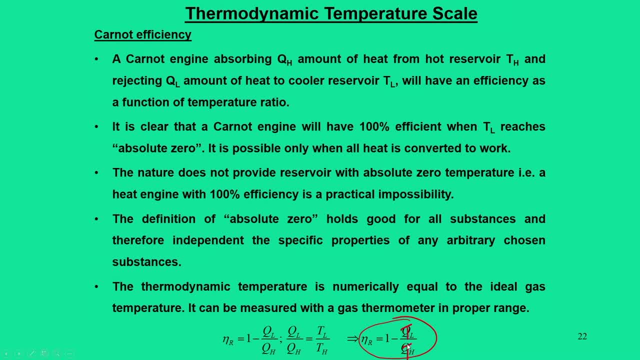 the temperature has to be expressed in a absolute scale. Now, in this equation, what we can say? T L goes to 0. when T L goes to 0, which implies efficiency of a reversible engine goes to 100 percent, And T L goes to 0 means it is a almost impossible situations, T L is 0. 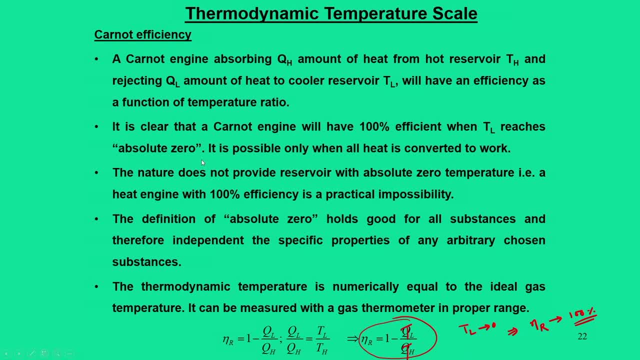 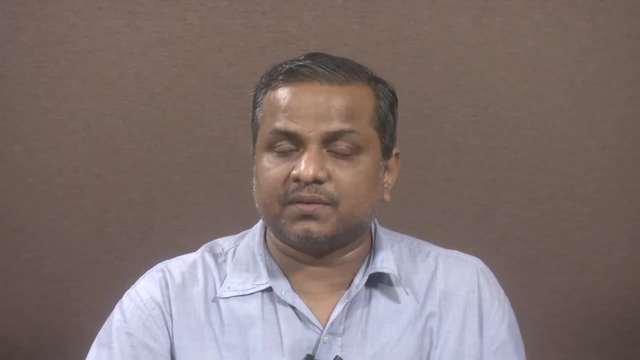 means we are going to absolute 0. So it is almost an impossible situations. So the Carnot engine can never have 100 percent efficiency. that means in other words T, L must have a finite value. Then if you go to the reverse processreverseconcept, then you can say that 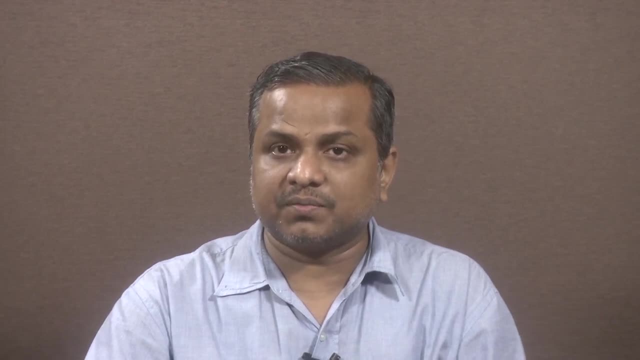 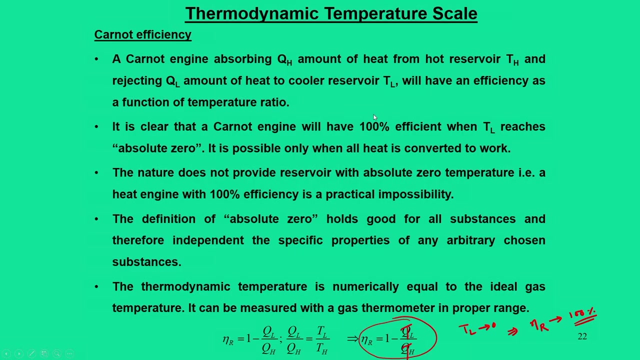 for from the for the conversion of heat to work is possible only when there is a rejection of heat to the low temperature sink. So the nature does not provide any reservoir with absolute zero temperature. that is, a heat engine with 100 percent efficiency is a practical impossibility. So the definition 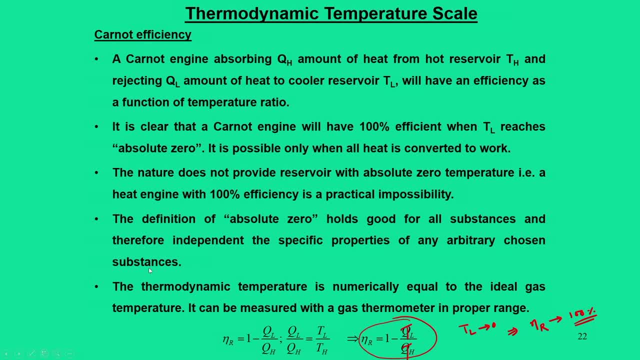 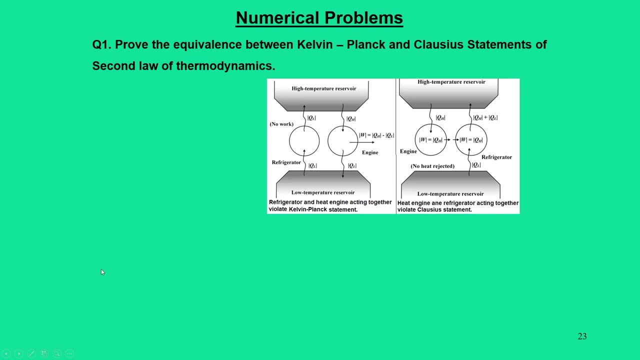 of absolute zero holds good for all substance and therefore it is independent of specific properties of any arbitrary chosen substances. So with this wecome to the end ofthis module 1, but before I conclude, I will just try to give some fundamental concept which are left out in this lecture. First, is that a proof? 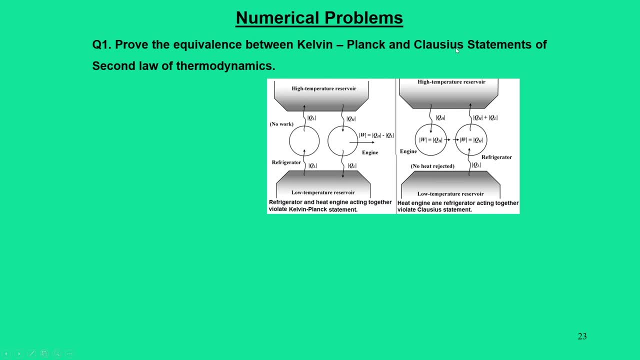 that prove the equivalence of Kelvin Planck and process statement of second law of thermodynamics. So I have already mentioned that if one of the statement is Invalid, that means if Kelvin Planck statement is invalid, other is also invalid. that means Clausius statement is also invalid. So to do that, let usrecall our figure which. 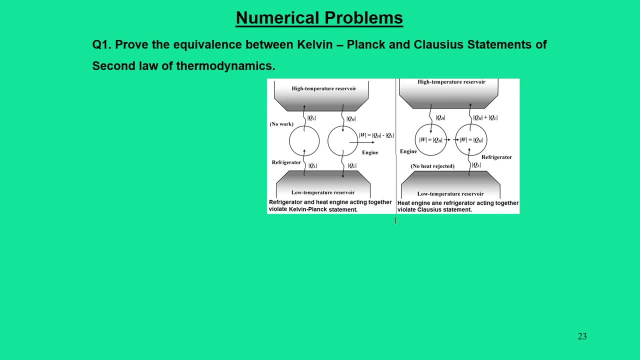 we have shown earlier where it is. it is said that it is said that in the firstcase we have this a refrigerator, and other one is unit, Another one is heat engine. So first of all, let me, let me put K as Kelvin Planck statement. 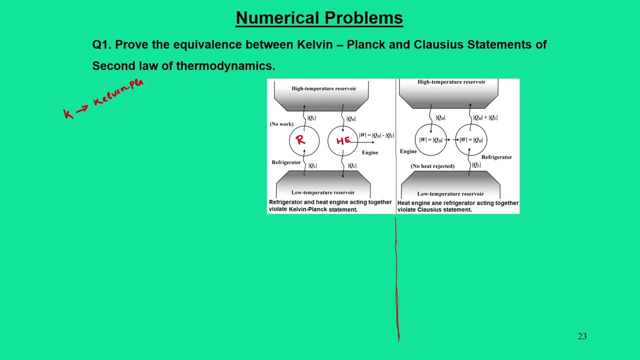 And if it is false then I will put it as a minus K. So that means if the Kelvin Planck statement is false, I will write it as a minus K. Similarly, C stands for Clausius statement, So I will put minus C as false if it is a 거. 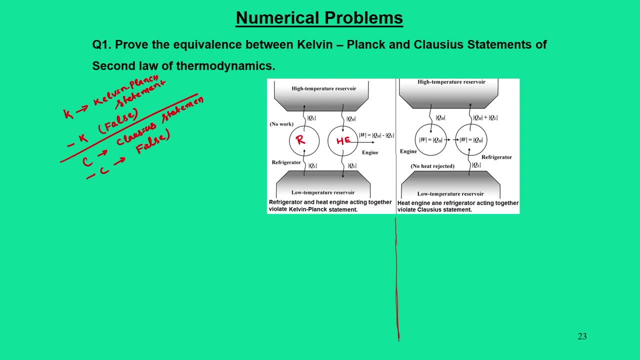 if the Clausius statement is false, is not satisfied. So since the second law of thermodynamics is the negative statement, So will try to interpret: if A, K is minus C, if K is 1, K is, if you try to interpret equivalence between K and C. in other words, I can say: if K is true, 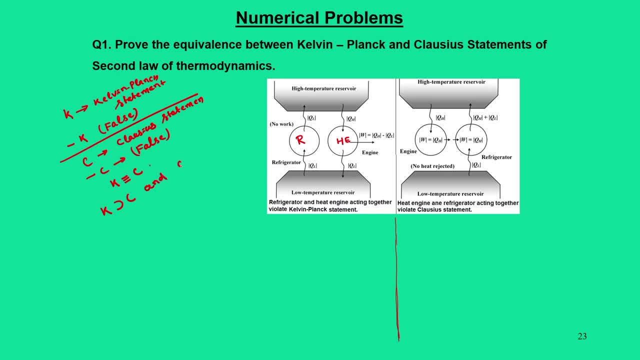 then Clausius statement is also true. Otherwise, if K is false, then negative value statement of Kelvin statement is false, then Clausius statement is also false. So all thesethings should also hold good. So this is true statement and this is false statements. ok, and this has. 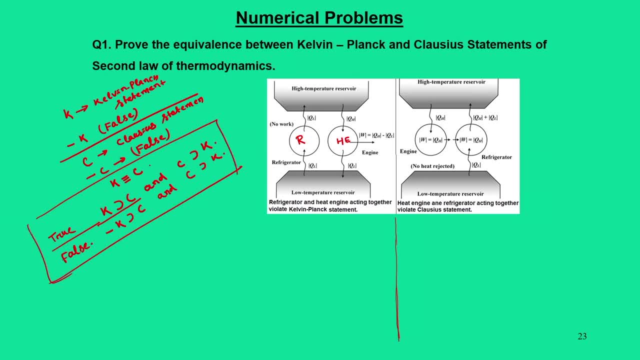 to be proved And which we call as As equivalence between Kelvin, Planck and Clausius statements. So first thing, we consider a refrigerator that takes Q, L amount of heat and also rejects Q L amount of heat to the high temperature reservoir, and in this process it does no work. That means we can say we 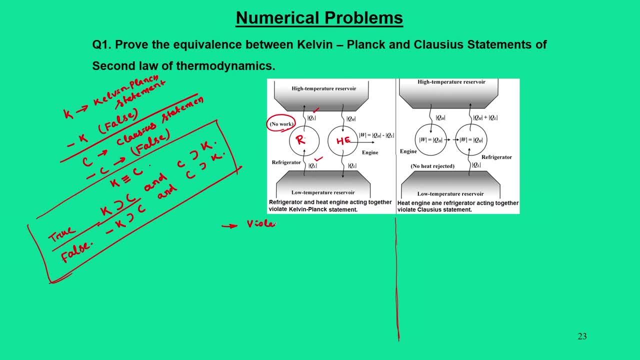 are now violating the violation of Clausius statement, So I will put it as minus C. violation of Clausius statement means it is minus C. Then we can for the in the same concept, with between samehigh temperature and low temperature reservoir, we are putting an heat engine that. 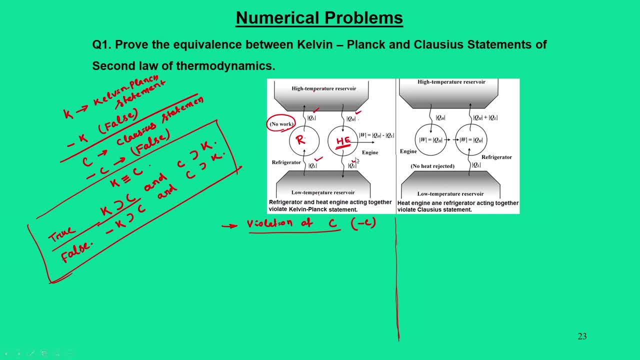 takes Q H amount of heat and rejects Q L amount of heat heat. So that means rejects Q L amount of heat to the low temperature reservoir And as a situation we say operation of heat engine, which is true Now, but globally. if you see, if you take both refrigerator and 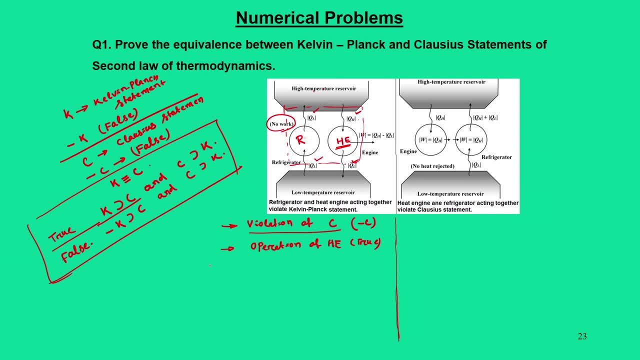 heat engine together. what you view is that combined machine takes Q h minus Q L amount of heat and produces W amount of. that is nothing but Q h minus Q L amount of work, but while doing so it does not reject heat. So this means it is. 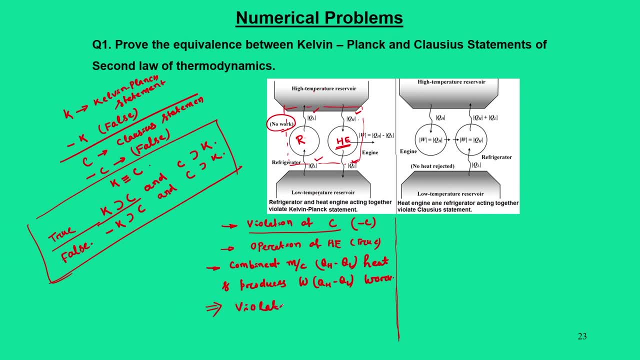 a violation of K that is minus K. So in other words it says that violation of Scorcher statement also is the violation of Kelvin Planck statement. In a similar logic we will put in a reverse way. that is, let us see that we have a heat. 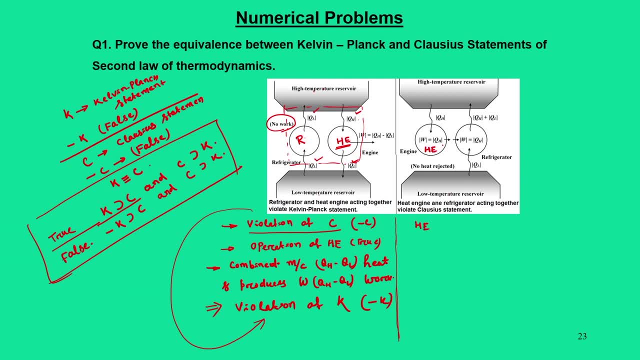 engine that takes Q- h amount of heat, but no heat is rejected. So for this, which means no heat rejection, means value rejection. So this can be done by this way And we have a heat engine that takes Q h amount. 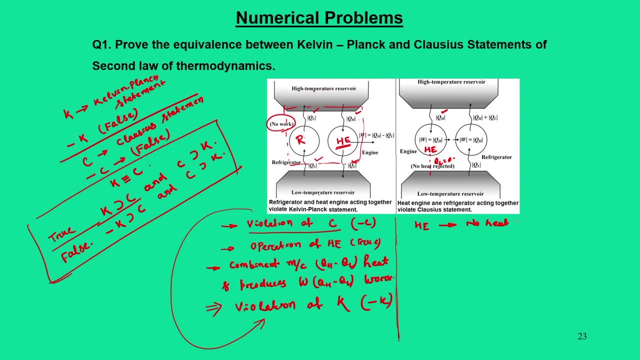 of heat, but no heat is rejected. So for this, which means no heat, rejection means value. a violation of Kelvin Planck statement means violation of Kelvin Planck statements, So I will put it as minus K Now. while doing so, we can also think about another refrigerator. 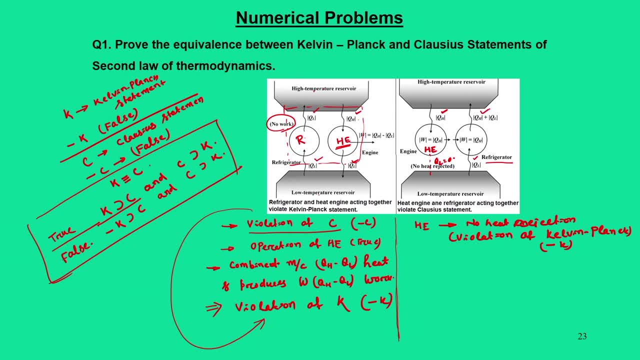 which takes q l amount of heat and rejects q h plus q l amount of heat to the high temperature reservoirs. Now in this process, if you join both heat engine and refrigerators- so we say that then we have operation of refrigerator. 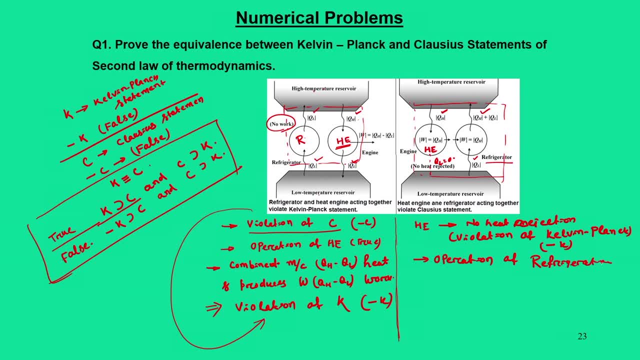 Ok, Ok. Ok Then for combined system: it takes Q L heat, does W arc and reject Q H plus Q W. So this, this will imply violation of Clausius statement. So from this we can say we started with violation of Kelvin Planck statement. we proved that. 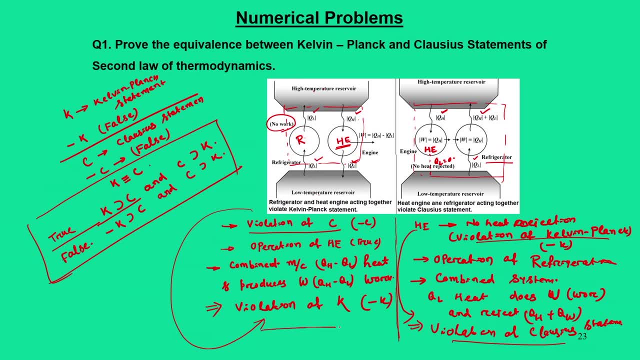 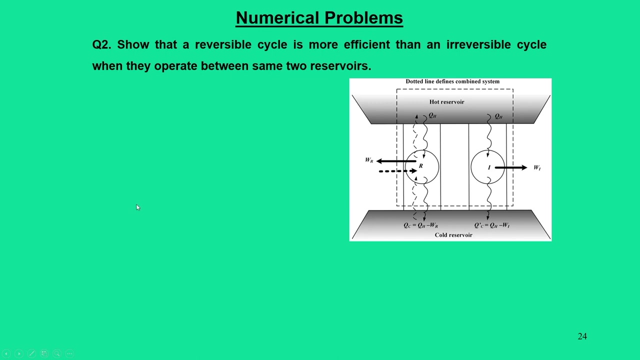 violation of Clausius statements. So, in other words, these two possibilities is never possible When these negative statement is proved. in other words, there is a equivalence between Kelvin Planck and Clausius statement. K is equal to K is equivalent to C. Now, in another similar problem, one of the corollary of Carnot cycle is that the reverse 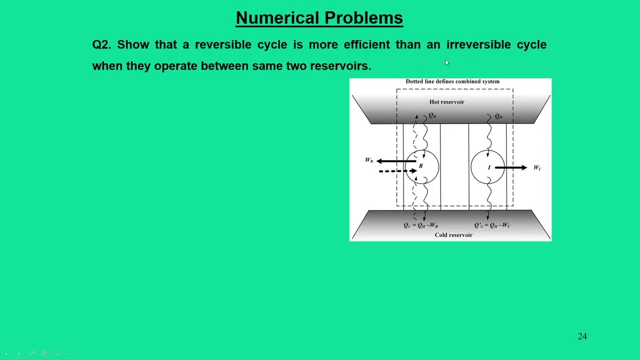 always a reversible cycle is more efficient than irreversible cycle When they operate it in same two reservoirs. Now to prove that we can say: we assume that there is a hot reservoir which is at temperature T h and there is a cold reservoir which is 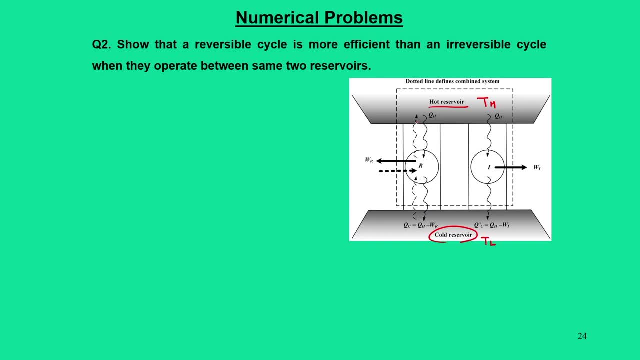 at temperature T, L And in between. we can imagine that there ispresable engine r and there is a irreversible engine i. When I say reversible engines, the, the heat transfer is Q? s and heat rejection is Q? q. cheat transfer from hot reservoir is Q? s and heat transfer from theto the low temperature. 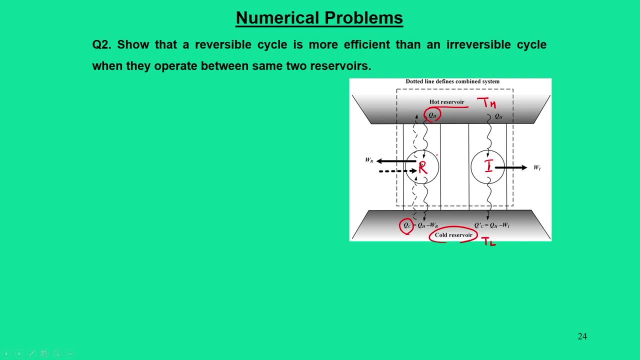 reservoir is Q, L And the both. the process is possible. eitherwe can give W? r amount of work to this reversible engine. take heat Q c from here and reject Q h to here. Other way, in heat heat engine mode, the engine can operate with W? r amount of work while 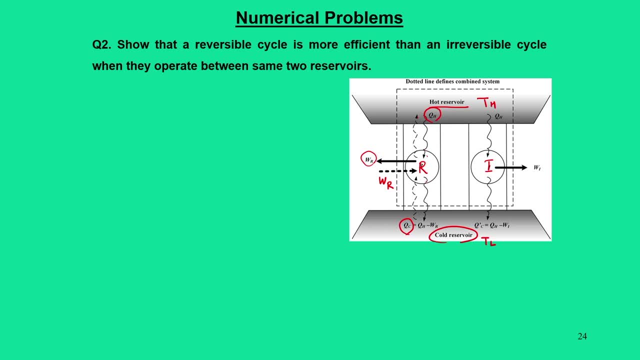 taking Q h amount of heat from the source and Q- L amount of heat, Q c amount of heat to the sink. So this is how a reversible engine operates. but in any reversible engines we both. this system is not possible. So I can say it only gives in one mode, that is, we get W? i amount of work while taking. 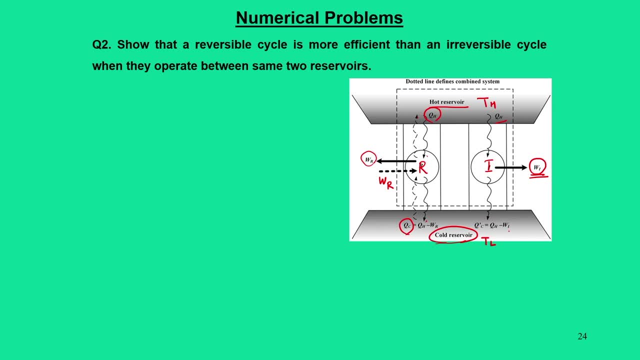 heat: Q? h amount of heat and rejecting Q dash h amount of heat to the sink. So in so in since these arereversible and heat reversible engines to. to prove this, to prove thisfact that reversible cycle is more efficient, then we have to recall the 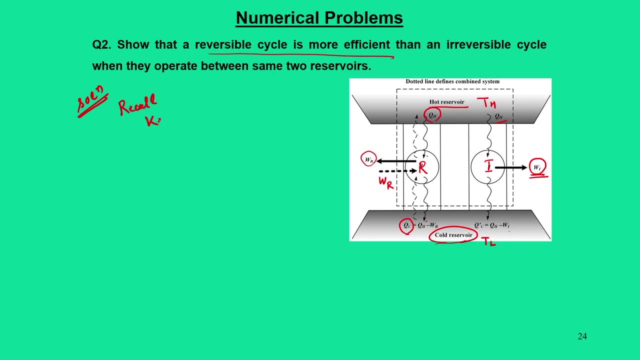 relation of this Kelvin Planck statement. This Kelvin Planck statement in a mathematical form, we write that W cycle is less than 1 or equal to 0. Now, in this, when you apply this particular concept, when for a combined system which includes this reversible engine and irreversible engines, 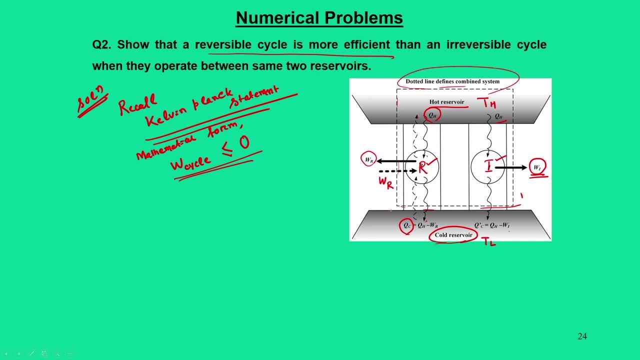 we can view this through a dotted line. with of this combined systems, We can write: w i minus w r is less than 0, because entire dotted line systems is nothing but is irreversible. And so we can write: w i is equal to w i minus w r is equal to 0. So in other words, 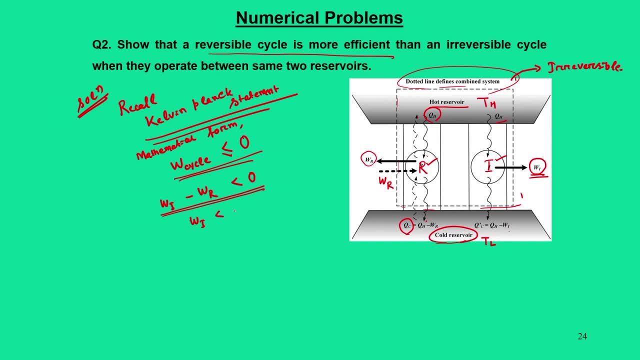 we can say w? i. that means work transfer in an irreversible engine is always equal to less than work transfer in the reversible engines. So from this, this is the proof, but what we have asked for: efficiency. So we can rewrite this expressions like, if you: 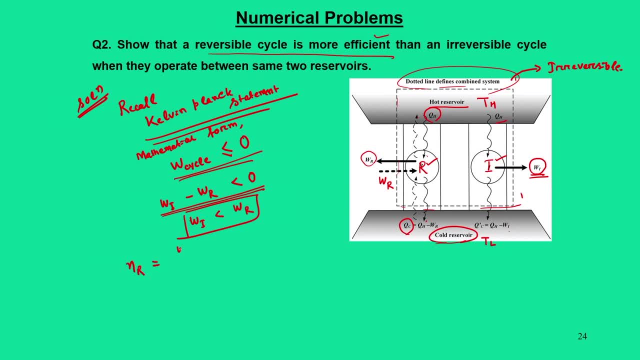 say reversible engine w r, we can write w r by q h and irreversible engine, eta i is equal to w i by q h And they q h is same for both the cases, So and w i is less than w r, So it means reversible. 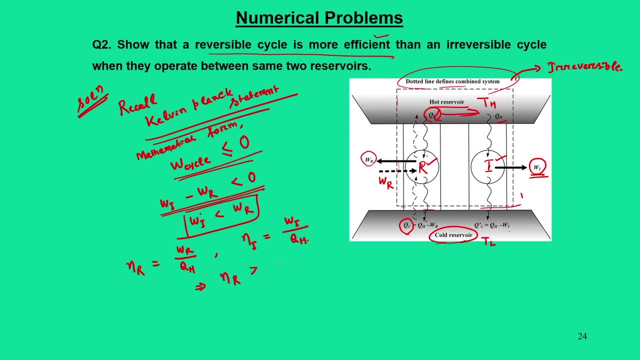 engine is has higher efficiency than irreversible engines. Another concept, that is first statement. Second concept would be that ifwhen we say reversible and irreversible engines, they, if both, are reversible engines, then we can say: w r 1 is equal to w r 2.. So assume that i is replaced with w r 2 and r is reversible. 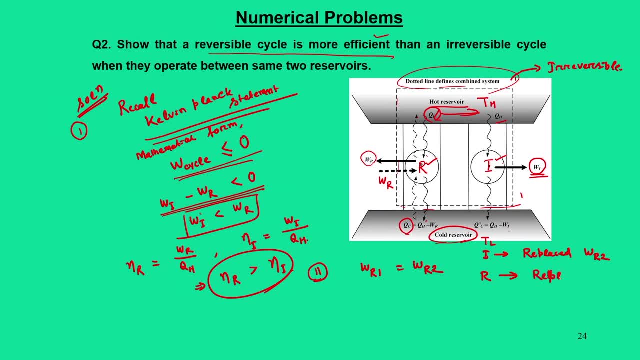 engines is replaced by w r 2.. W r 1. What we are trying to prove is that if the both the engines are reversible, then the efficiency of reversible engine r 1 is also equal to efficient efficiency of the reversible engine r 2. Which means all the reversible engines operating between same. 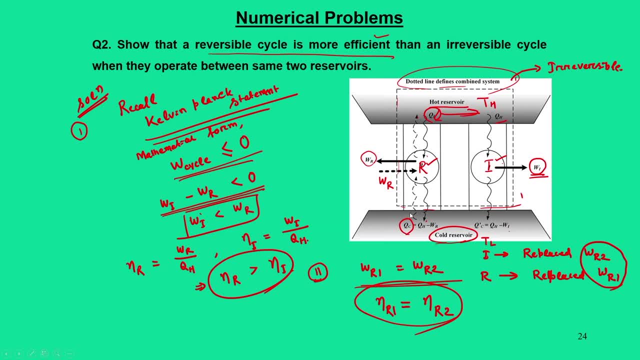 two temperature limits are half same efficiency. that is first with this second statement. So statement First statement was: if reversible engine has always higher efficiency than the irreversible engines. So these two statements are nothing but corollary ofsecond law of